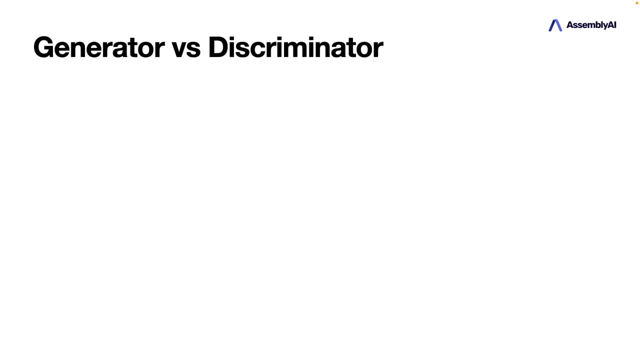 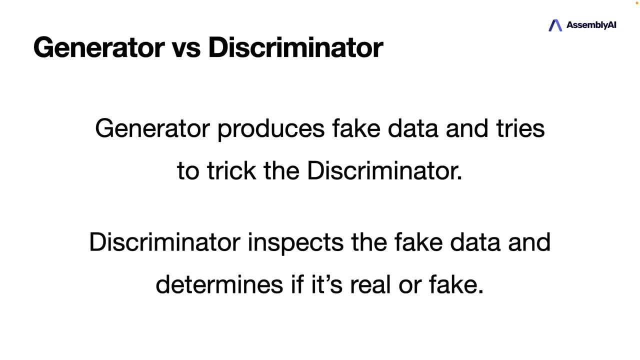 other. So how does this work exactly? So the two networks are called the generator and the discriminator. And the generator produces fake data and tries to trick the discriminator, And the discriminator inspects the fake data and then determines if it's real or fake. So this is like a detective, And then they play against each other. So this is. 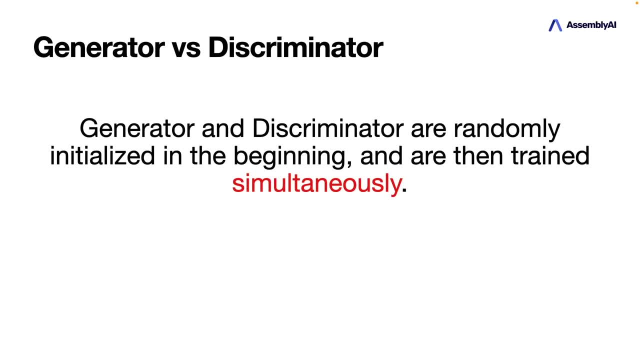 basically the training. So first they are initialized randomly and then they are trained simultaneously And this means we have to minimize two losses. So we also use two optimizer and we use the binary cross entropy loss. So I'm not going into detail here about the loss formula. 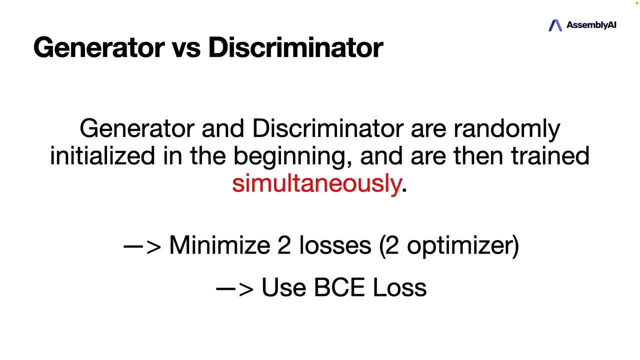 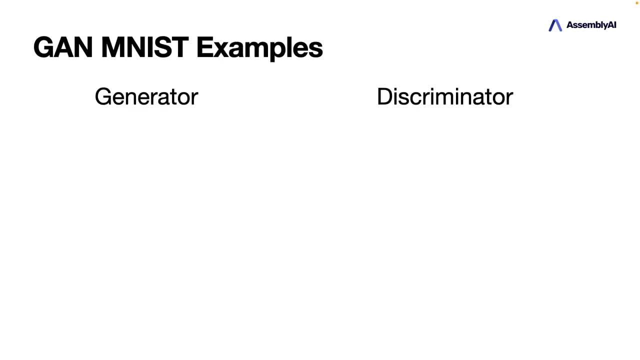 but I will link another resource below the video if you want to learn more about this. And yeah, this is basically the whole concept. And now, before we jump to the code, let's look at an example. So later we use the MNIST data set. So now the generator tries to. 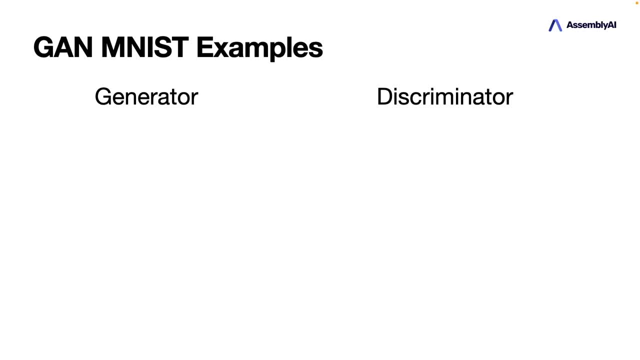 generate MNIST images. So these digits from zero to nine, and then tries to trick the discriminator, and then they play against each other and both sides get better and better. And in the beginning they don't know anything, So they are randomly initialized. So the 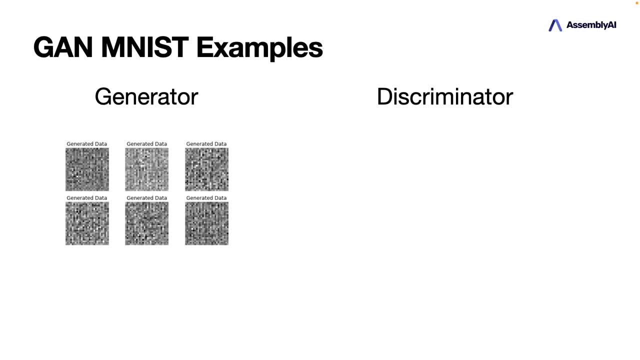 generator just produces noise. So random data that might look like this, And then the discriminator looks at this and can also look at real data and compare it, And then it might easily say, yeah, this is fake. But then the learning or the training continues And then the generator comes. 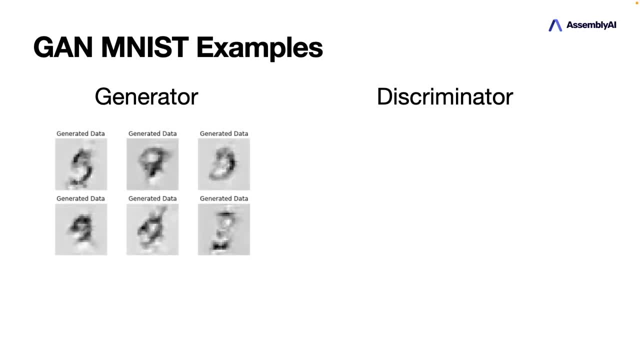 up with new data And this might look something like this, And then again the discriminator looks at it and it can simply still say: yeah, still fake. But then at some point the generator just produces noise. So random data that might look like this, And then the 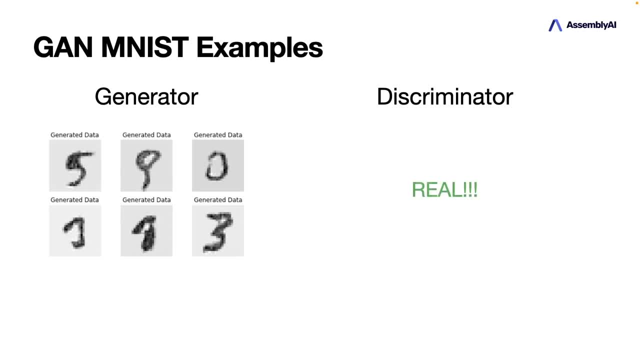 generator gets better and better And then the discriminator might be tricked and say: yeah, this is actually real data. So obviously in this example the data is still not perfect, But of course also the discriminator is still not perfect, So it also has to improve. 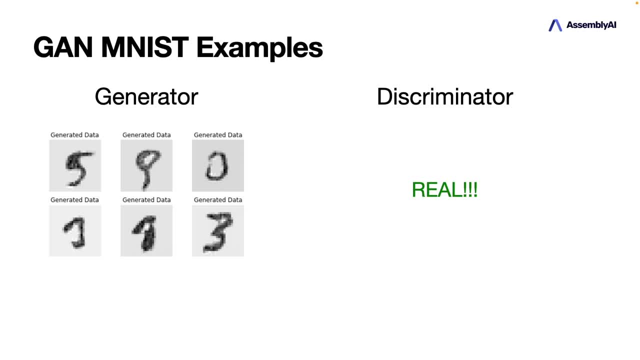 And then this continues and both sides get better and better And eventually we get a, or should get a- generated data that should not be easily distinguishable from the original data. And yeah, this is how it works. So now let's jump to the code and see how we can implement this. Alright, so here I'm, in a Google. 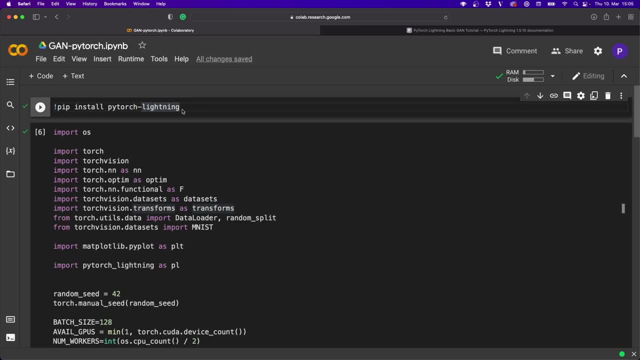 colab, And I already prepared some code for the start, But later we will write the rest of the code together. So I recommend that you just copy this colab into your own folder and then follow me here. So I will put the link in the description And the first thing you should do is set the 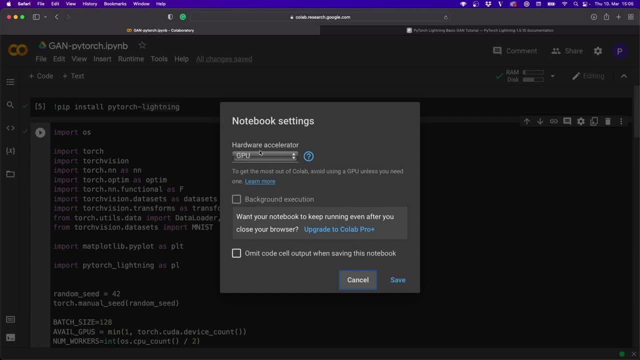 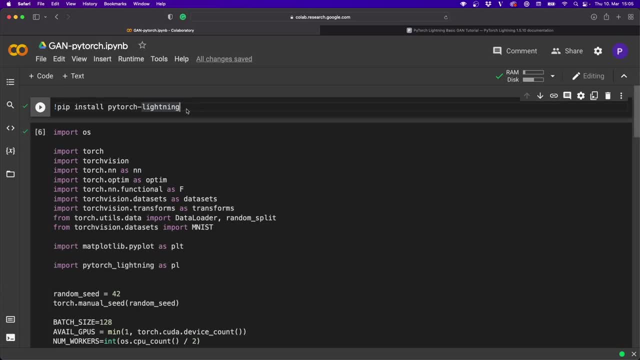 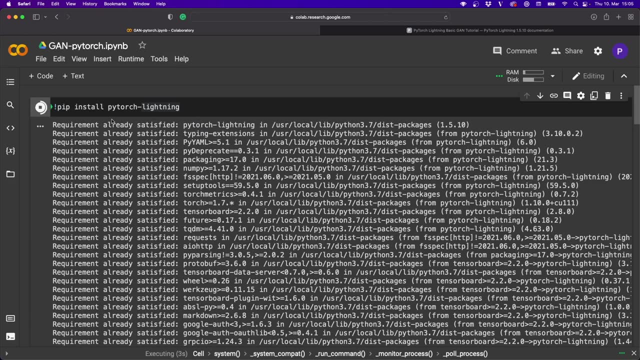 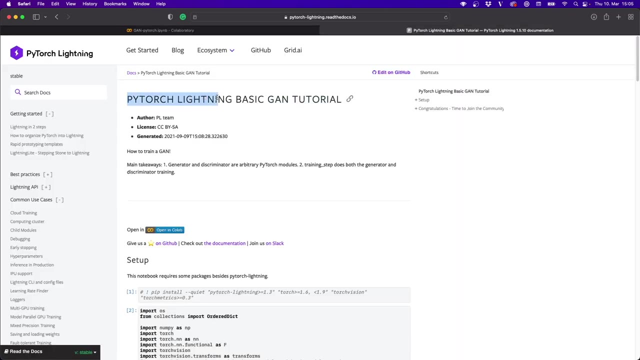 Then the training will be much faster. And then the first thing we do is we say: pip, install PyTorch lightning. because we also use PyTorch lightning here to make the code a little bit shorter. And I also want to mention that there is an official Gantt tutorial on the PyTorch lightning. 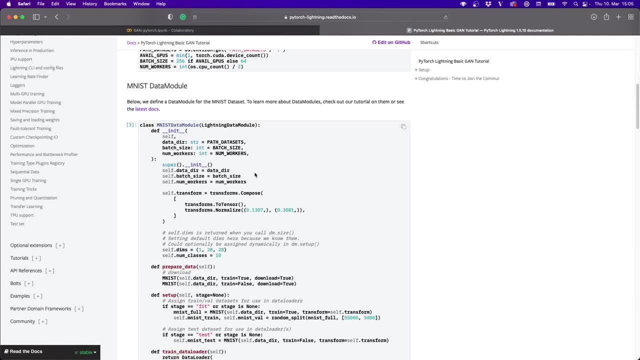 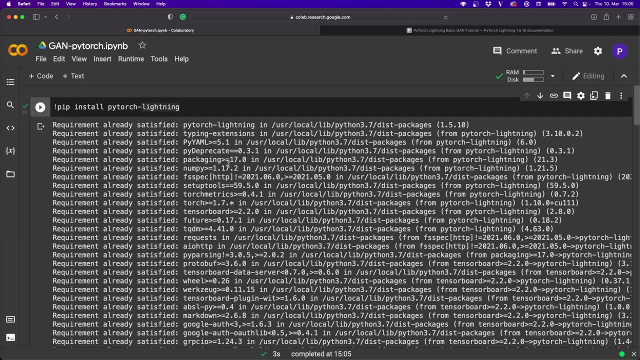 website That is pretty similar to my code, But in this case they just use normal linear layers And in our case we use CNN, And so it's a little bit different. But yeah, this is also a great resource that you should check. 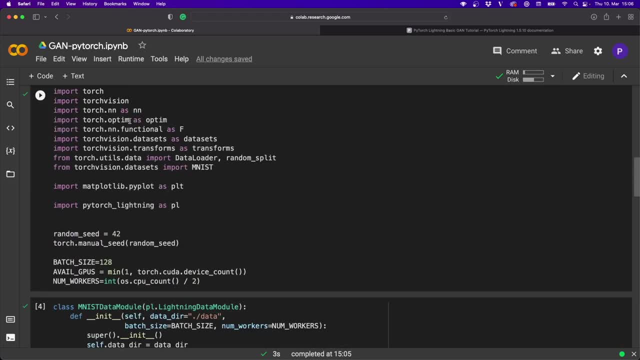 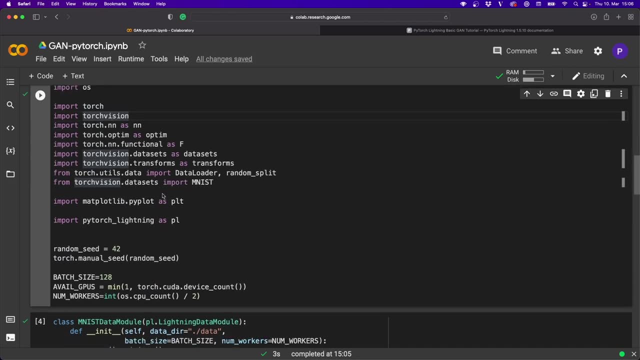 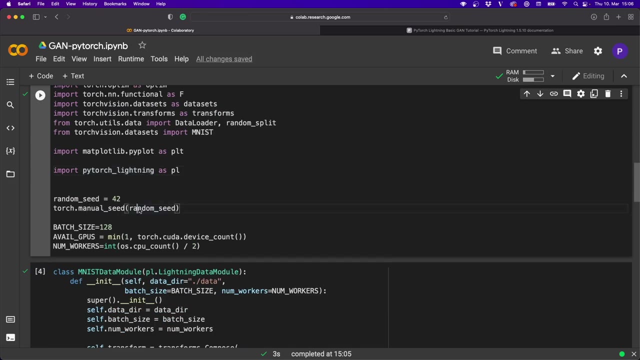 out. So yeah, we install this here. Then here we do all the imports we need, So torch and torch vision and the different modules. Then we also use py matplotlib and PyTorch lightning, And then here we set some parameters, for example a random seat, the batch size. we check if we have GPUs. 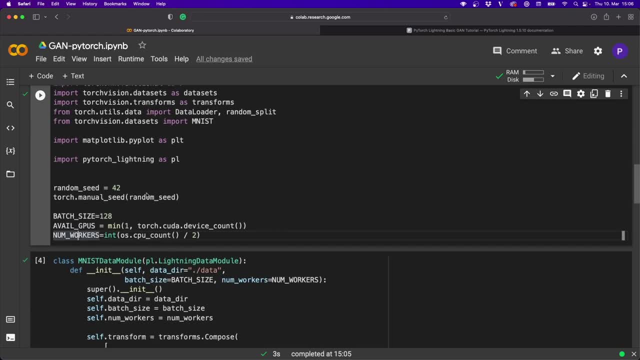 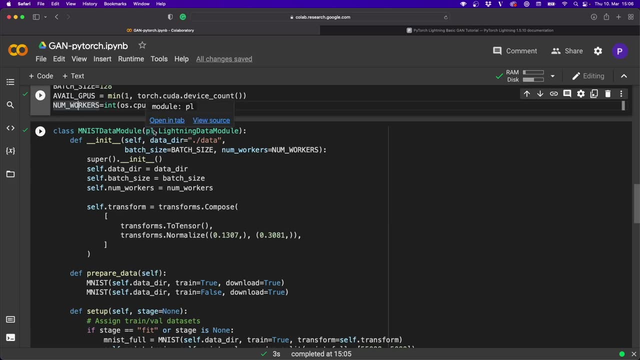 And if we have multiple CPUs, we check if we have multiple CPUs. And if we have multiple CPUs, we check if we have multiple CPUs. And if we have multiple CPUs, we check if we have multiple CPUs. And then the first thing we do is we create a data module that inherits from PyTorch lightning. 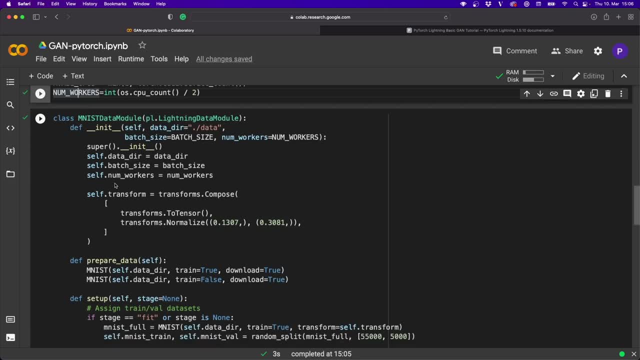 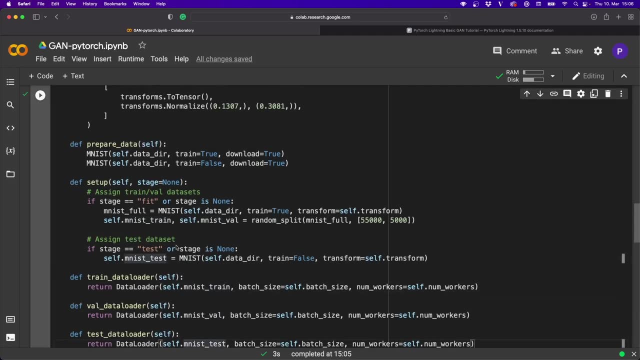 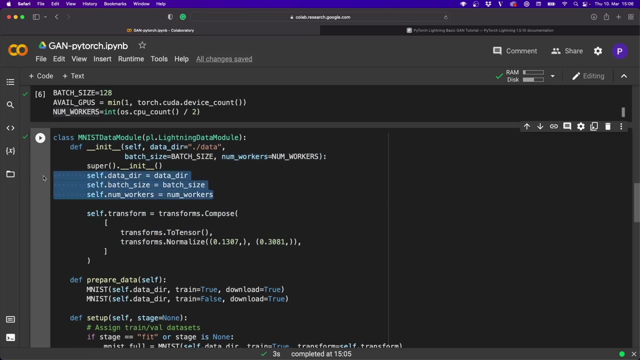 dot lightning data module. So this is responsible to create the data loaders for us for the training, validation and test set, And the way this works is that we have to implement the init function. So here we simply define the parameters And we also define the 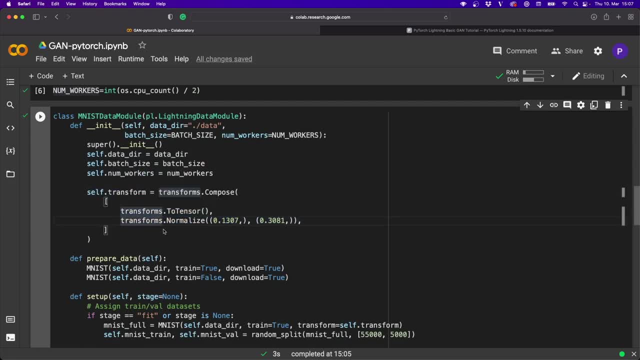 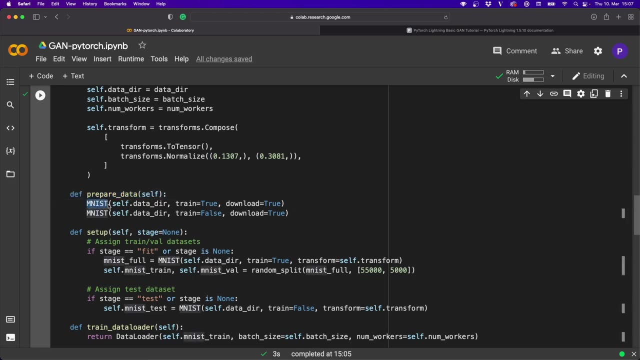 transformations. So here we convert from images to a tensor and then we normalize it. So this is the mean and the standard deviation from the MNIST images. then we have to implement the prepared data function. So here we call the built in MNIST data and we can set: download equals true. And then this: 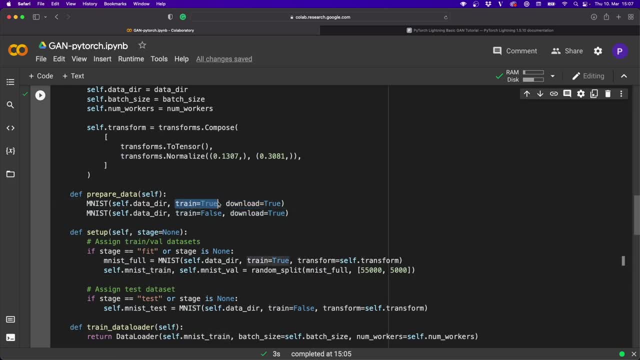 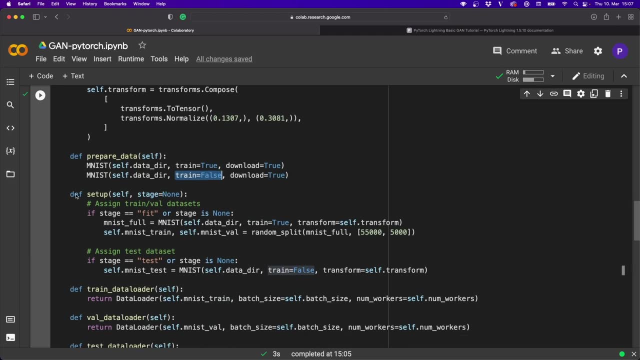 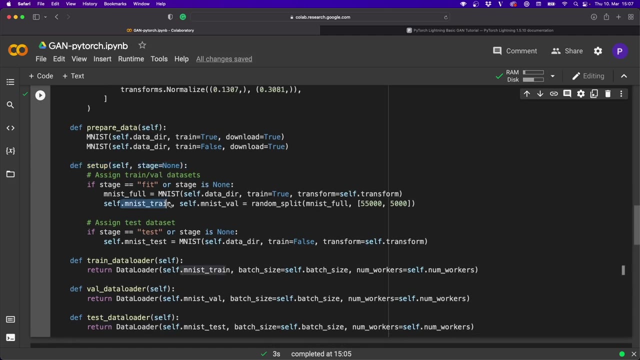 will download the data And one time we say training equals true for the training set, and then one time training equals false for the test set, Then we also implement the setup function. So here we further split the training data into training and validation set by applying this random split function. And yeah for the test set. 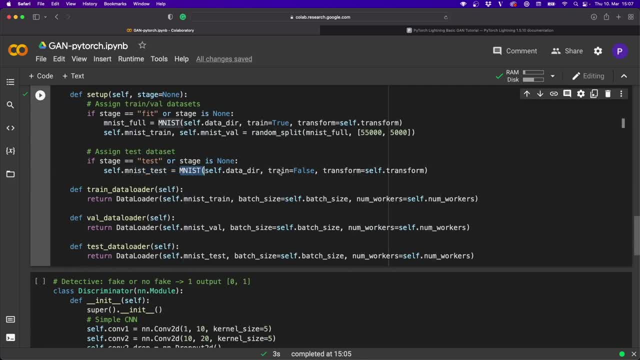 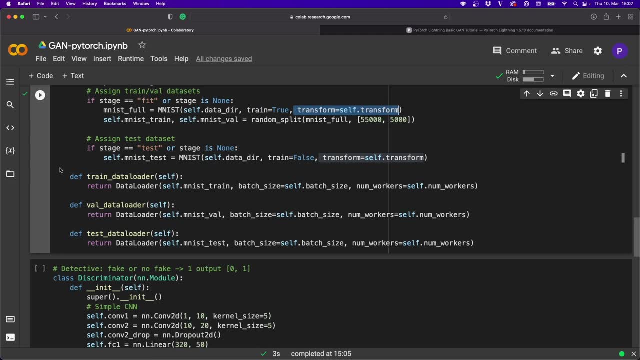 we simply also create the MNIST data by saying training equals false, And in all steps we already apply the transformations, And then we can implement these three functions to train data loader and the test data loader, And they are all pretty simple, So they just return the data loader with. 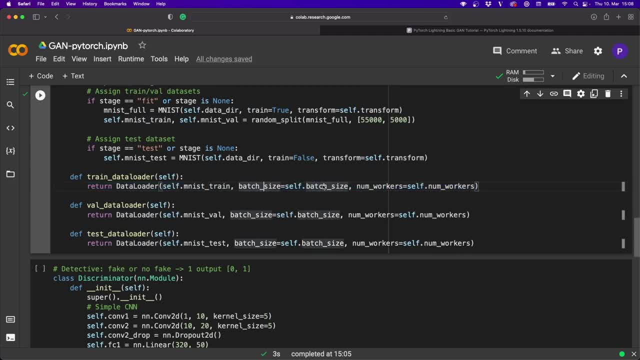 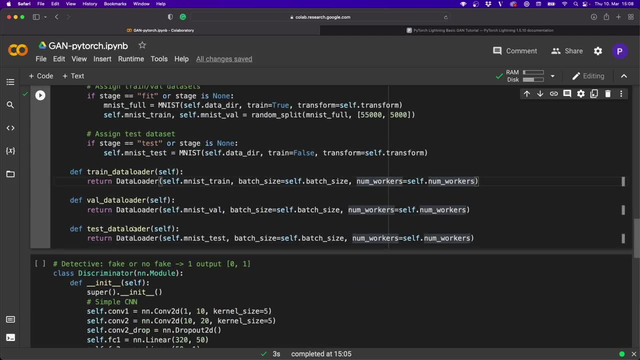 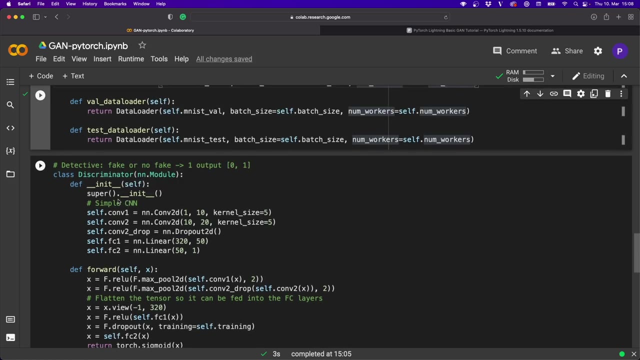 the corresponding data set, And then we can also set the batch size and the number of workers. So yeah, this is what we have to do: to get the data loaders, And then we have to implement the two networks, so the discriminator and the generator, And they are both vanilla pytorch. 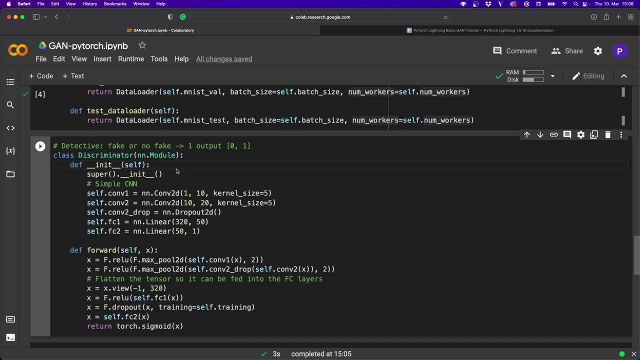 modules So we can mix and match pytorch and pytorch lightning. So for the discriminator we create a class that inherits from nn dot module And, like I said, the discriminator is like a detective, so it has the task to detect if it's fake or no fake. So in the end we only need 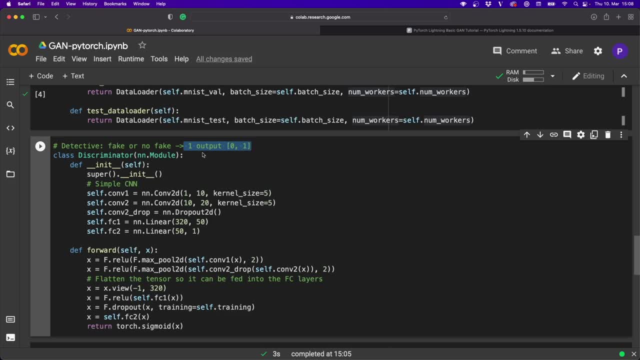 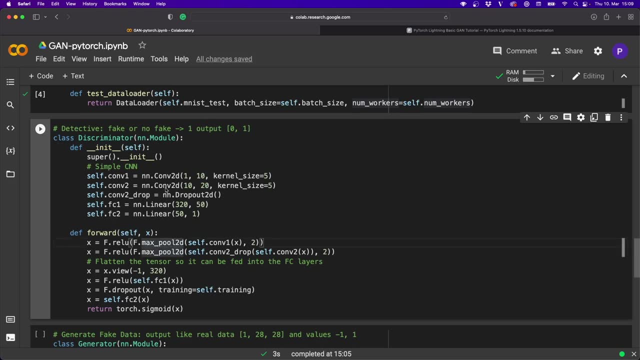 one output that must be between zero and one, And we only have to implement the init function and the forward function, And basically, here you could use the same function, but here you could do whatever we want, But in the end we only want one output that is between zero and one. 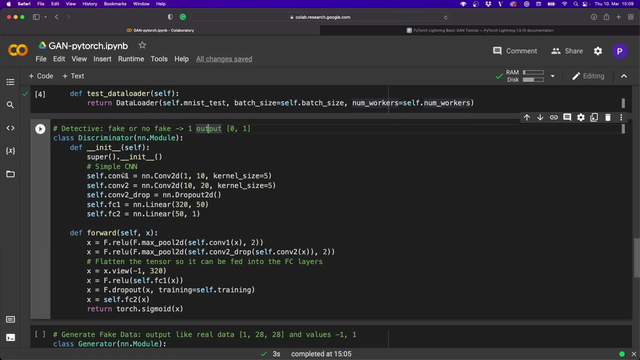 So you could just use linear layers. But in this example I want to show you how we can use CNN. So we use two convolutional 2d layers, then we also use a dropout layer in the 2d case And in the end we use two linear layers. And, yeah, we always have to be careful that we have. 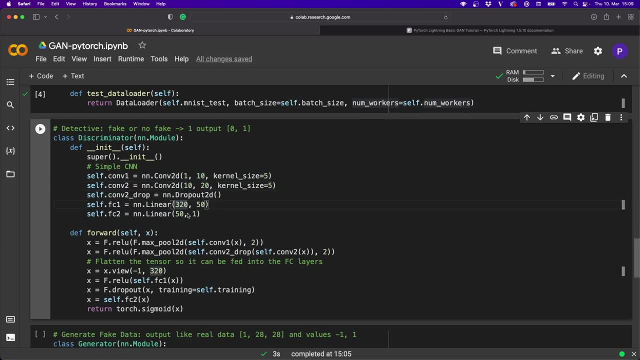 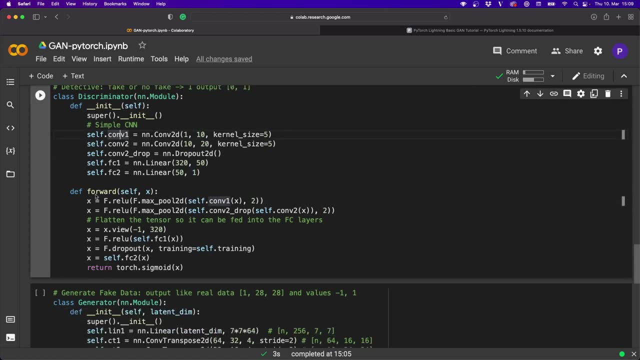 the correct input and output sizes. And then the very end, we need one output. So yeah, in the init function we simply create all the layers, And then in the forward function we apply all layers And we also apply max pooling and 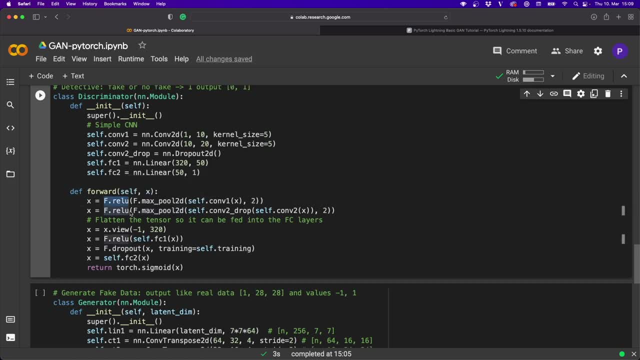 activation functions. So here the relu activation function. So yeah, first the first convolution with max pool and relu, then the second convolution with dropout max pool and relu, then we reshape the data so we can feed it to the fully connected layers. Then we apply the first fully connected layer, So the linear layer with an activation function. 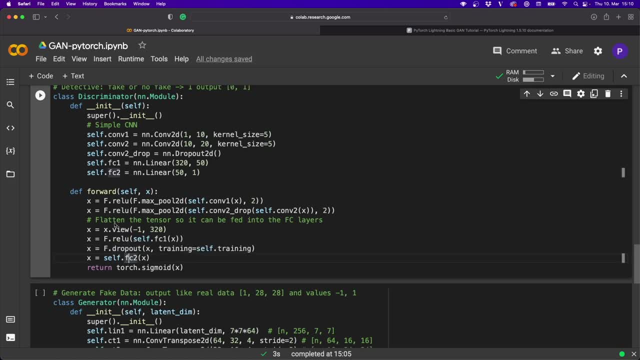 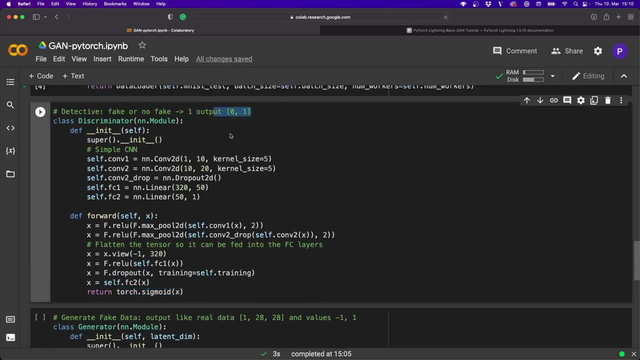 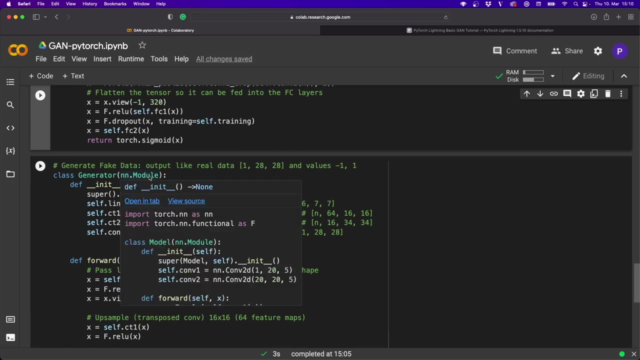 a dropout, and the second fully connected layer, And then, in the very end, we apply the sigmoid function. So this takes care that the output is between zero and one. So this is our discriminator. And now the generator basically works the other way around. 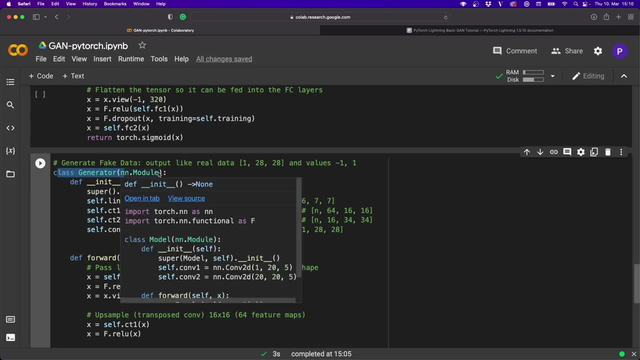 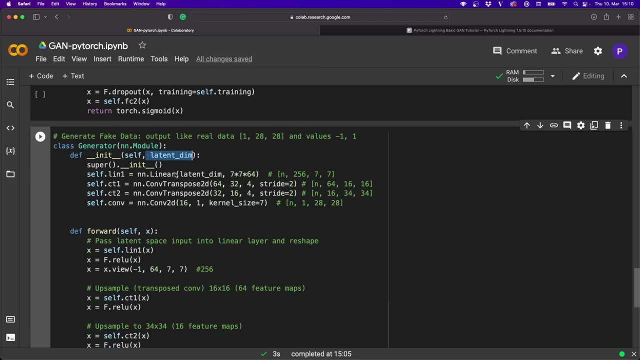 So we also create a class that inherits from nn dot module, And here this gets as a parameter the number of latent dimensions. So this is a scalar value, And basically from this value we up sample to a output that is in the shape that the original images is. so 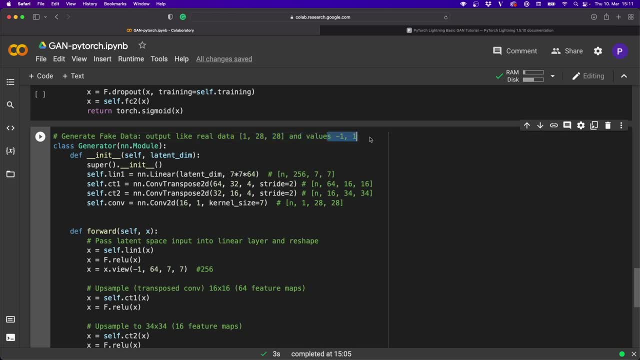 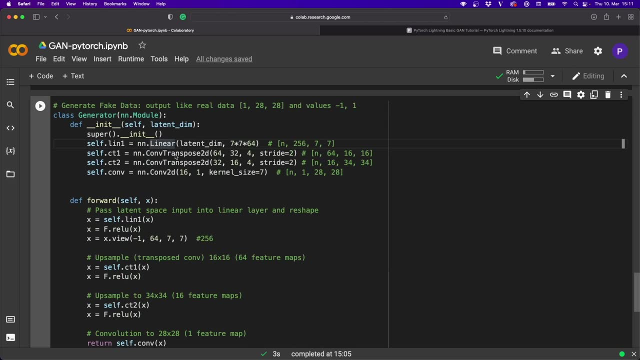 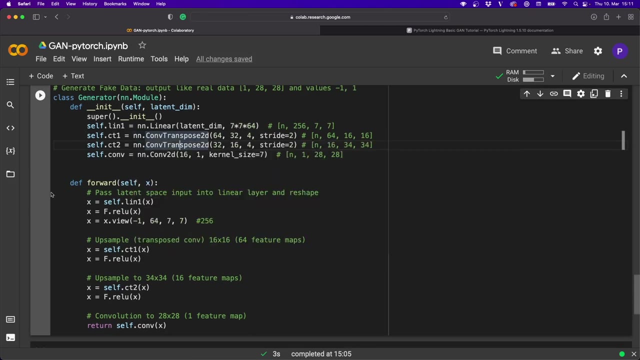 one by 28, by 28.. And the values are between minus one and one here. So here we also use a linear layer, then we use a convolution transposed to D layer, so two times actually, And then in the end we apply a normal convolution to put it back again into this shape, And then in: 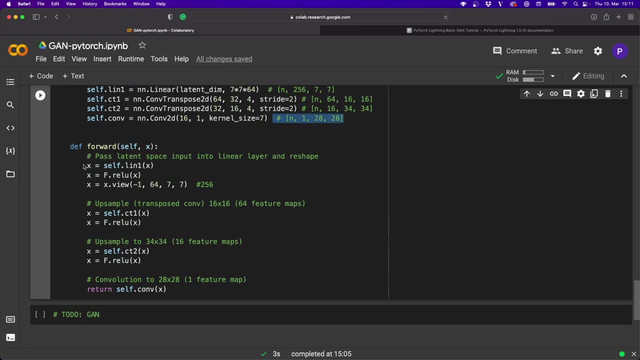 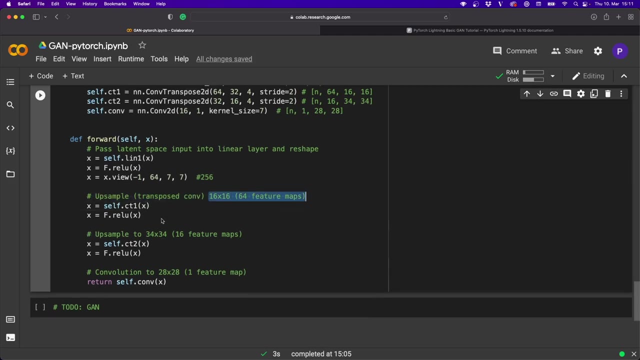 the forward pass. we apply all these steps. So first we apply the linear layer with a relu activation, then we reshape, then we apply the convolution transposed layer. this will up sample the data to be in this shape. then again a activation function, then the second convolution. 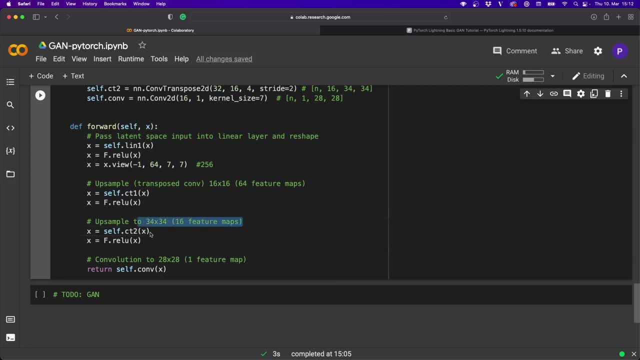 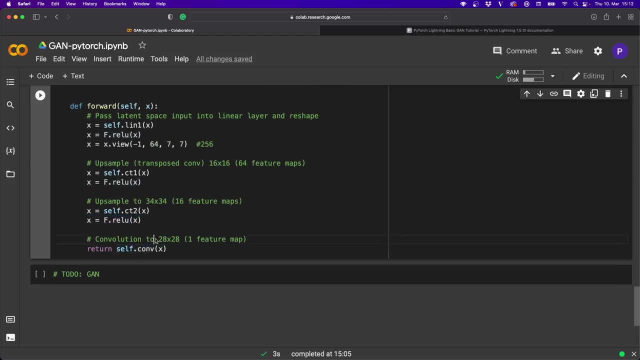 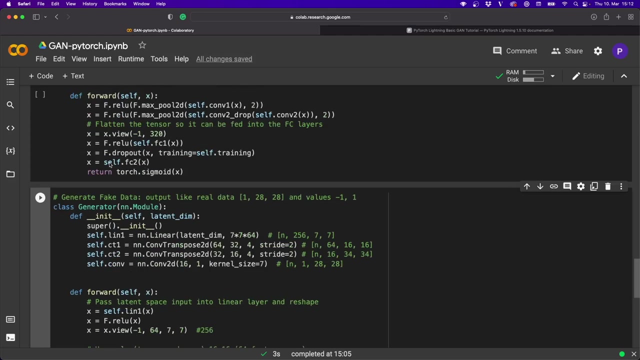 transposed layer. this will put it into this shape, then again a activation function and, at the very end, a normal convolution, which will put it back into this shape and then no activation at the end. So yeah, this are. these are the two networks that we need, And now we put them together in one. 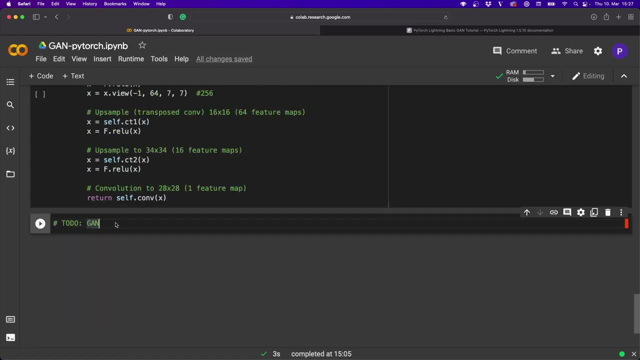 one class. So let's do this together. So here we want to create one class that we call again, and this inherits from pytorch lightning, dot lightning module, And then we have to implement a few functions so that it works with pytorch lightning. So first of all we need the init. 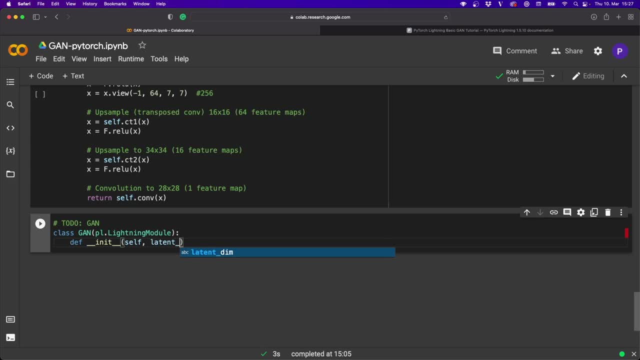 function with self, and then we also give it the number of latent dimensions, and this should be 100 by default. And then we also give it the number of latent dimensions, and this should be 100 by default. Then we also give it a learning rate, And by default, this is 002.. So you might actually want. 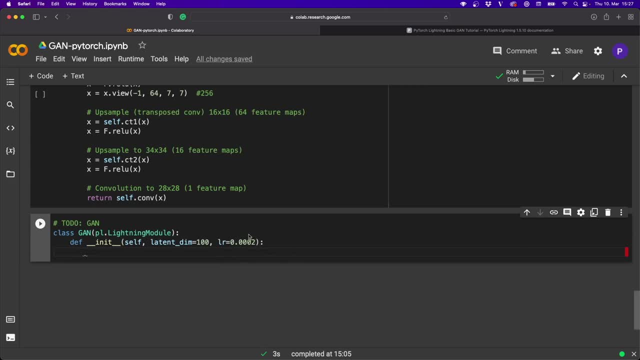 to play around with this a little bit. So it's very the learning is very sensitive to the learning rate, So it's very important that you have find a good one here. So yeah, by default, just try this one. Then the first thing we do we call the super initializer. So super in it like 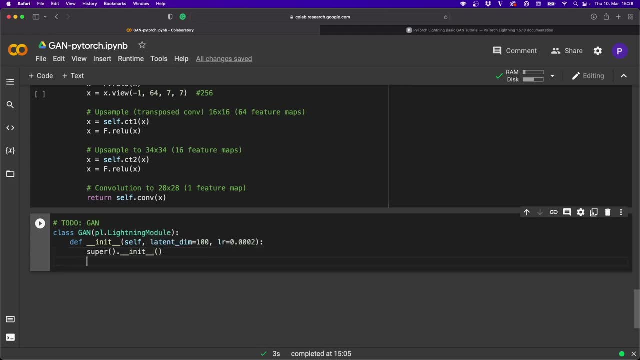 this. And then here we store our first, save the hyper parameters. So we say self dot, safe hyper parameters. this will make it accessible everywhere later. And then we create our two networks. So we say self dot generator equals the generator network And this gets one parameter. this is the latent dimension, equals. 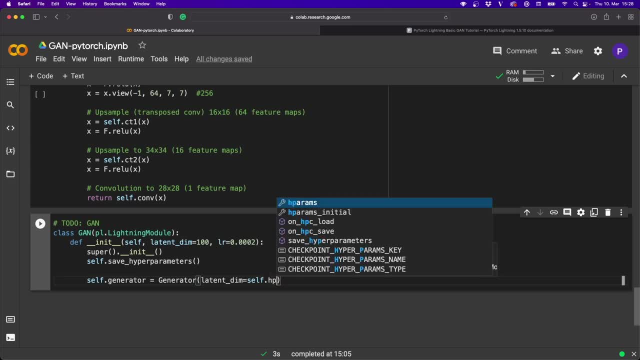 So we can access the hyper parameter by saying self dot, HP, params, dots, And now we can use latent them. So this is the same name that we use here for the parameter name. So this is our generator. And then we do the same thing for discriminator. So we initialize a discriminator. 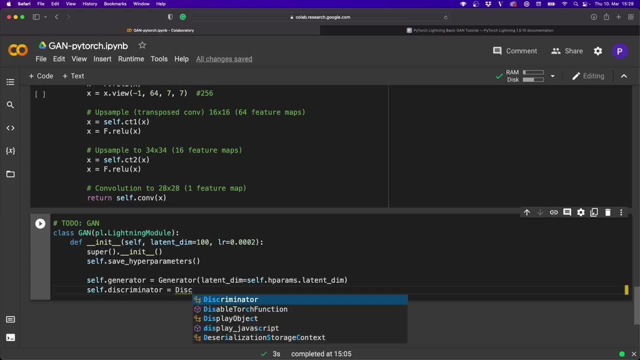 by saying this is a, this criminal, And this doesn't get any inputs. And then we create a random noise that we want to use later to test the images. So we say: self dot validation c equals torch dot rent n, And then it should be. 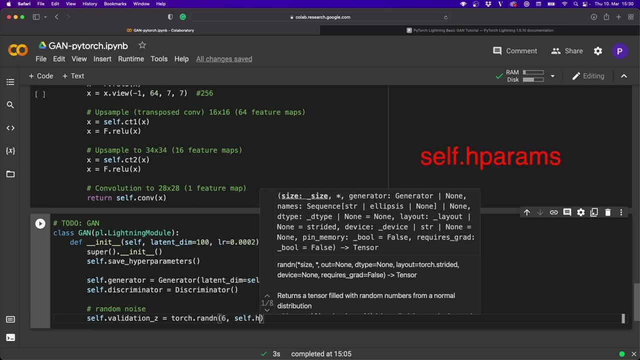 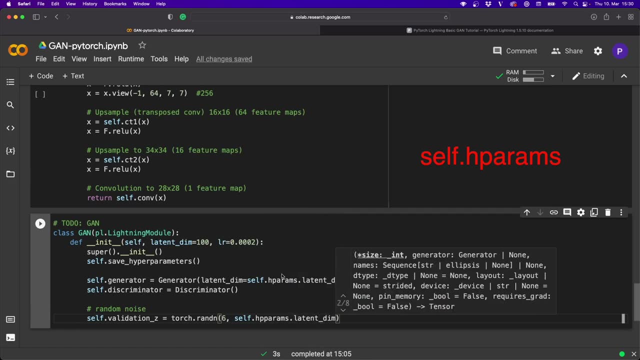 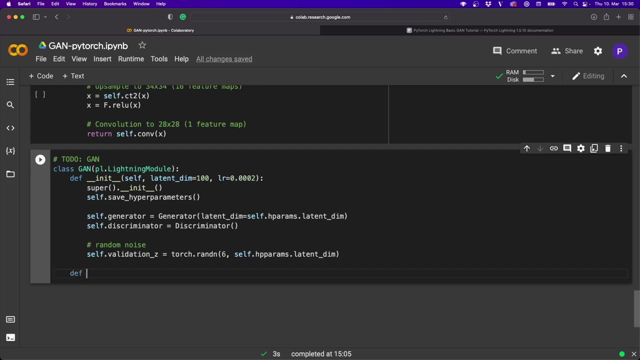 six images And we use self, dot, HP, params, dot, latent, underscore, dim For the second size And yeah, this is the init function. then we need to implement the forward function which gets self and the input tensor. So we call this C And the forward pass in the GAN. 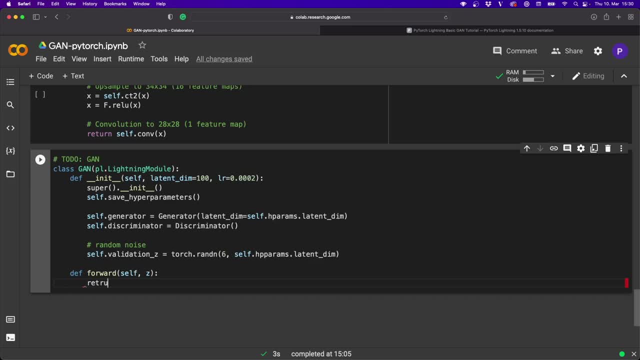 is actually just the generator. So here we can say: return self, dot Jenner rater, And this gets the input, the tensor as a input. So this is the forward pass. then let's create a function to define the loss. So we call this adversarial underscore loss, also with self, and then it gets y hat. So the predicted 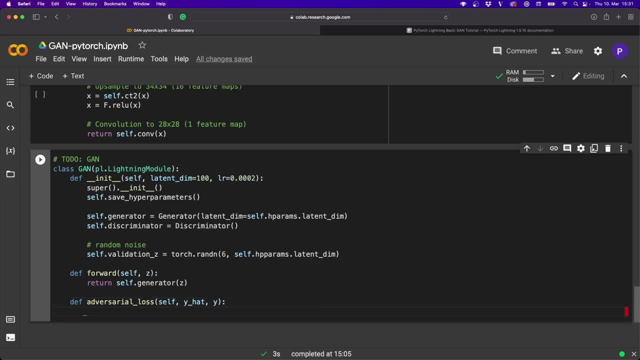 labels and the actual labels. And here we, as I said in the beginning, we use the binary cross entropy. So this is just a one, one liner. So we say: return f dot, binary cross entropy. And then here we feed it with y hat and 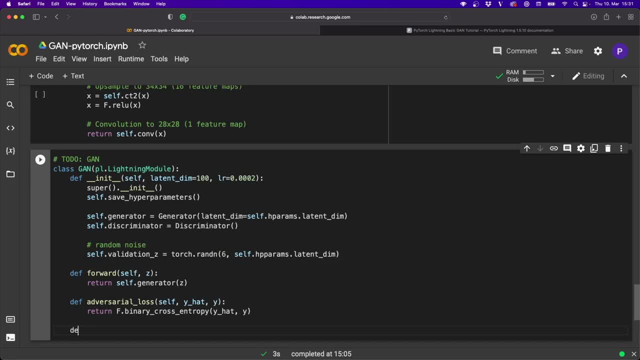 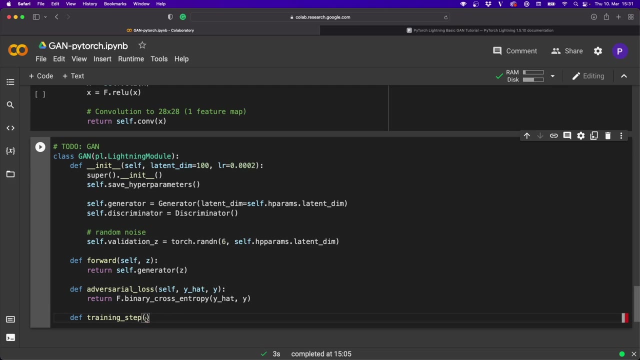 y, then we need the training steps. So define training steps. So this is actually a function from pytorch lightning that we have to implement And then everything later will be taken care of for us. So this gets self, then it also gets a batch, then it gets the batch index And it also gets the 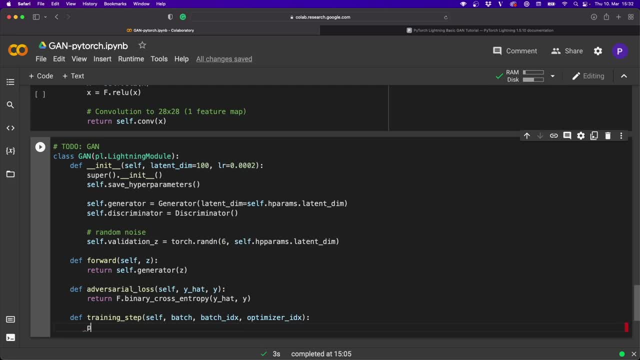 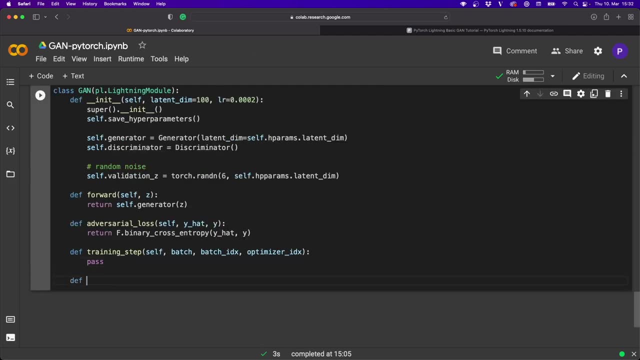 optimizer index And for now let's just say pass, So we do this as last step. then the next function we have to implement from pytorch lightning is the configure optimizer function, and this only gets self and it's actually called configureoptimizer. 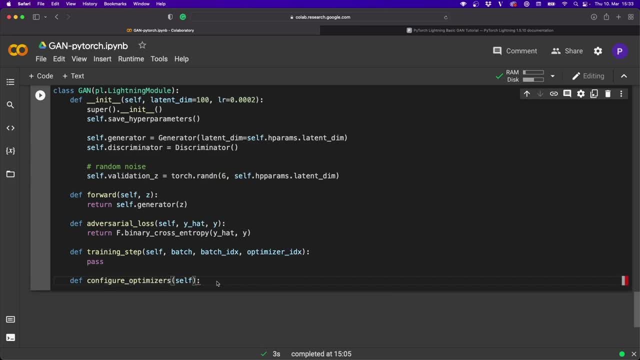 And then it'll come back from python the next time we're done with. I'll say find, then we also do this as last step. Then the next function we have to implement from pytorch lightning is the configureoptimizer, called configure optimizer s optimizers, And here we can access the learning rate by saying: 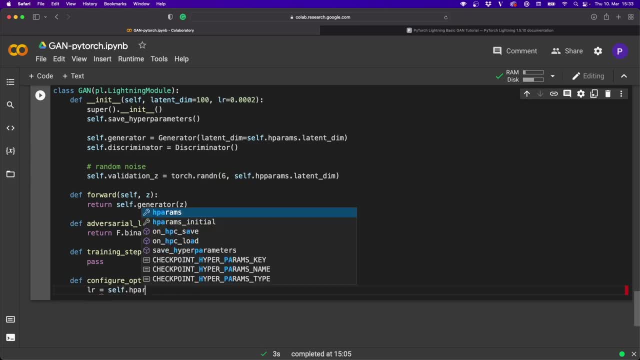 l r equals self dot h, params dot l r and then l r, And then we create two optimizers, one for the generator and one for the discriminators. So we say: opt G equals, And here we say: torch dot, optim dot Adam, for example, which is always a good choice. And then we want to: 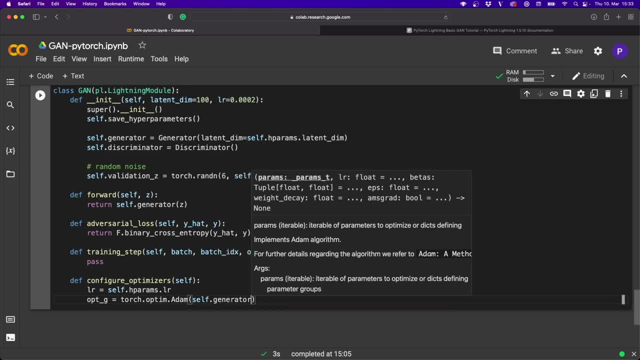 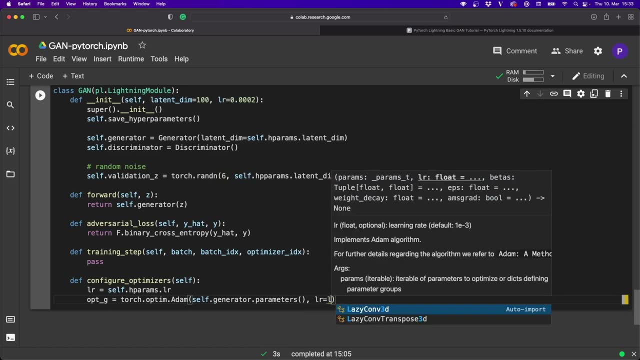 optimize self dot generator dot parameters And we also give it the learning rate. l r equals l r. Then we copy and paste this and do the same thing for the optimizer for the discriminators. So opt D, And here we minimize self dot discriminator dot parameters And we use the same learning rate. And then 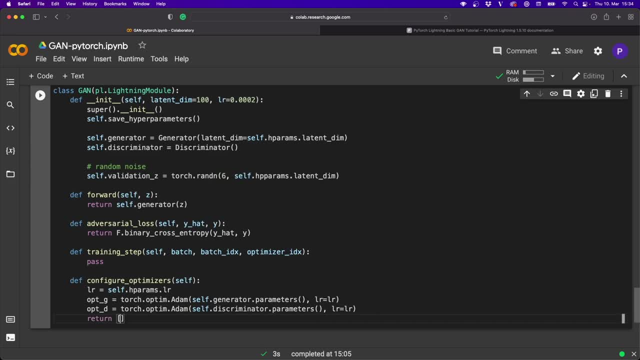 we return those. So we say return and then as a list, opt underscore G and opt underscore D And as second parameter we return a empty list. So this would be if you use a scheduler as well. And then there is one more function that we want to implement for the pytorch. 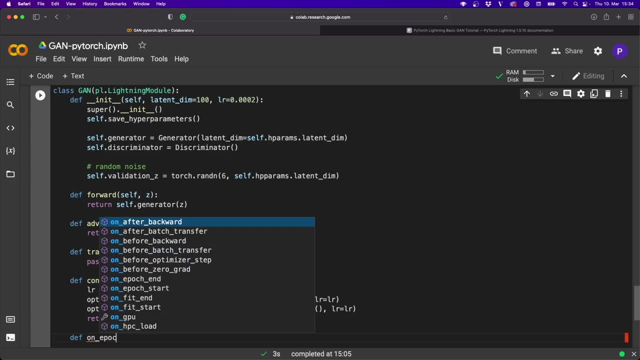 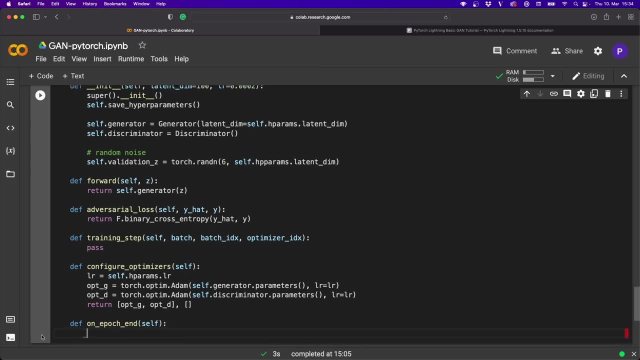 lightning module. So this is called the on epoch and function. This also only gets self, and here after each epoch I simply want to plot a few generated images to see how our fake data looks like. So here I call self dot plot images And this is a function that 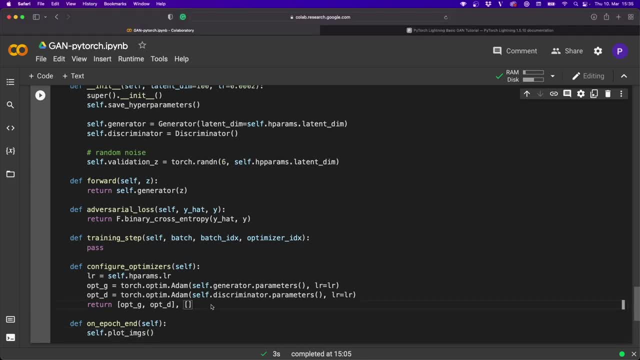 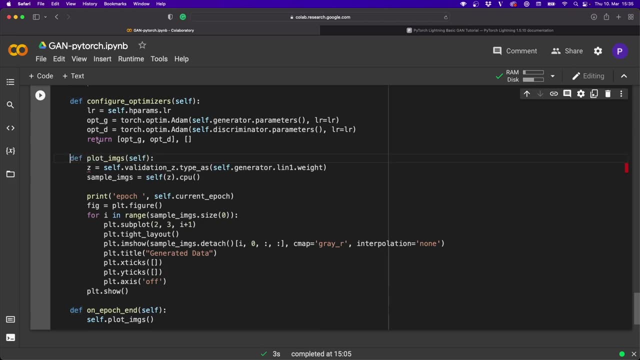 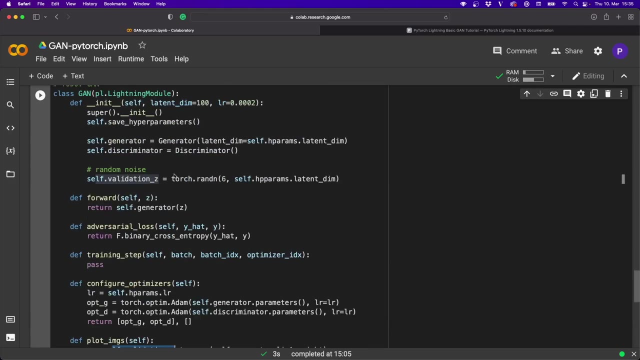 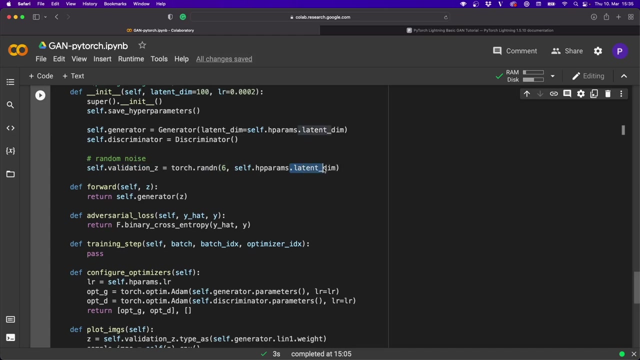 I simply copy and paste for you. So let me copy and paste this in here. So this will be one function, And what we do here is: here we use this validation, see that we created up here. So this is a random noise with six images and this number of latent dimensions. 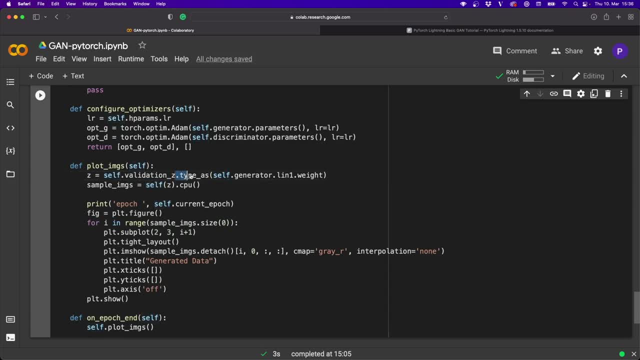 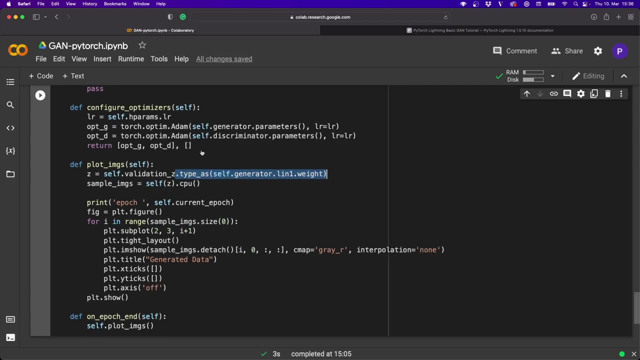 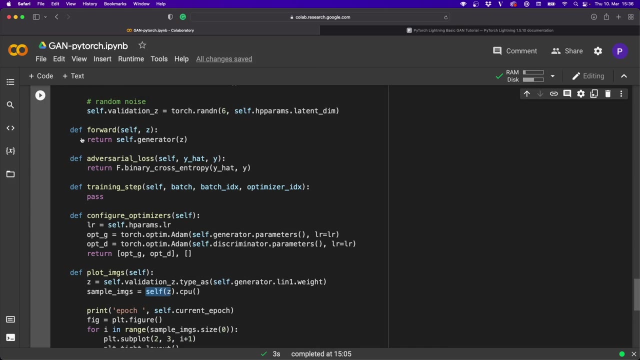 So here we use this and then we also use this type s function. this will basically move it to the GPU or not. if we don't use a GPU, then we call self dot C, So self dot C will execute the forward pass. So this will. 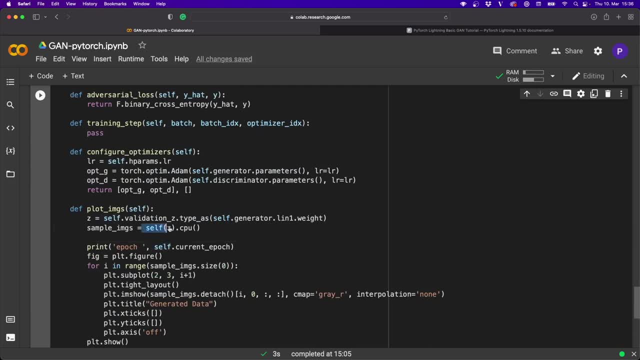 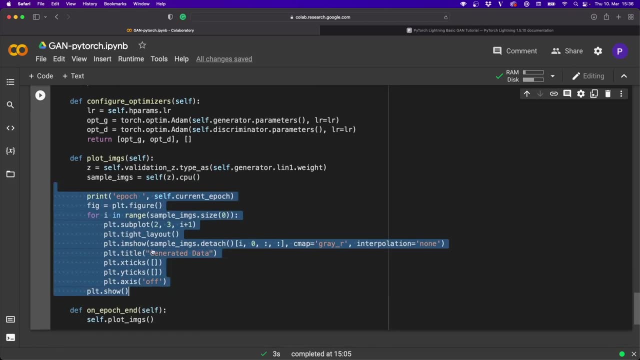 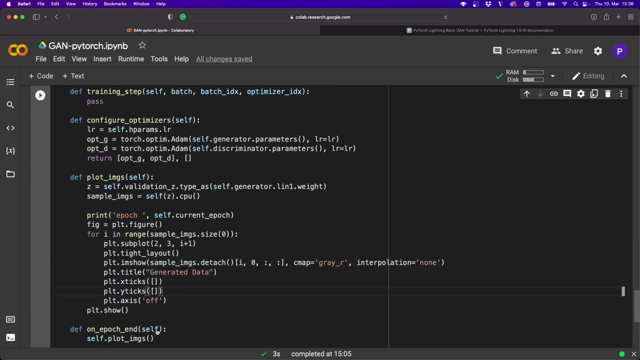 execute the generator, So this will generate some images, and then we put it back to the CPU And then here I have a small code snippet to generate some images with my matplotlib And then plot this as a grid. So yeah, this is what we do after each epoch. 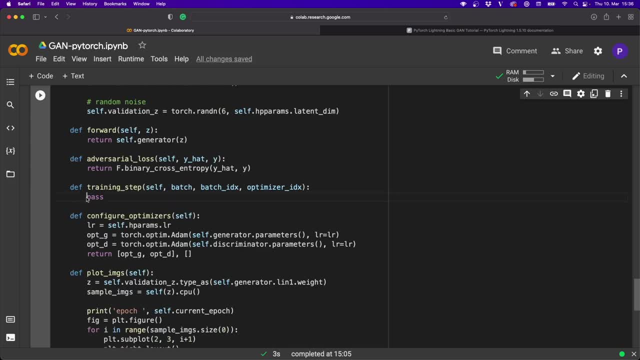 And now the only thing left to do is to implement the training steps. So let's do this. So here, First of all. here I noticed I have a typo, So this is just self dot h params. And yeah, now let's do this. So here, first we want to unpack the batch, So we call this the real. 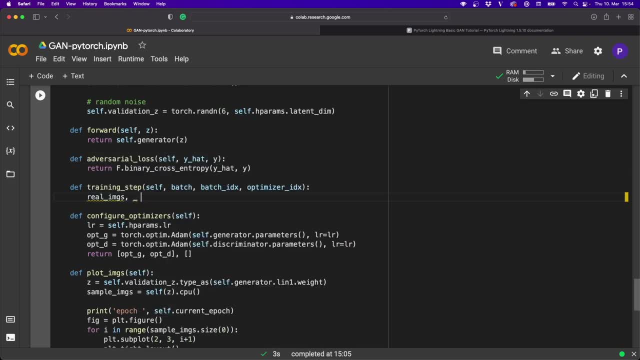 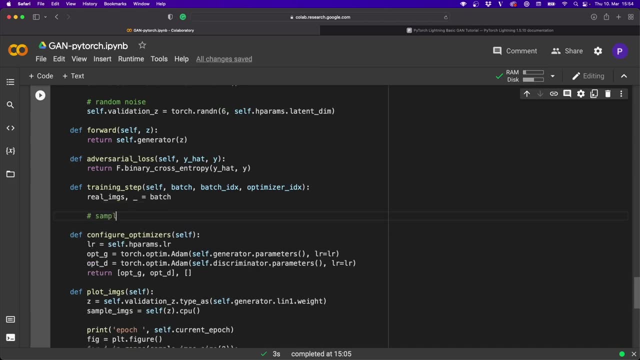 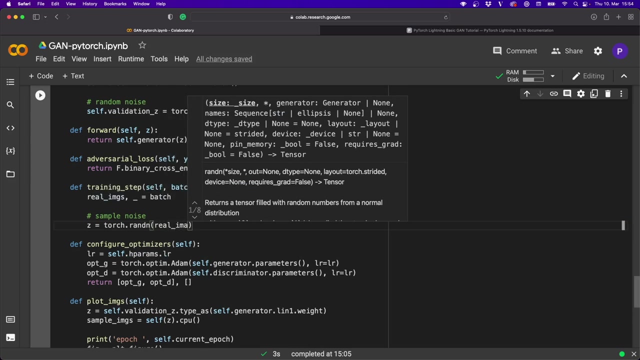 images And then just an underscore, because we don't need the labels, And this comes from the batch. And then again we create a sample noise data. So here we call this: C equals torch, dot, rent, n. And now it gets the shape of the real image: E, M, G, s. and then the first dimension, zero. 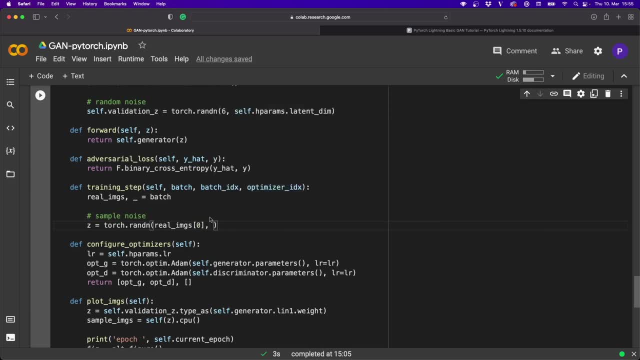 And then the second number, it gets the number of latent dims. So self dot h, params dot, latent dim. And then we again have to move it to the GPU if we use one. so we say C equals C dot type underscore s, and then we want to use the same type as the image tensor. So 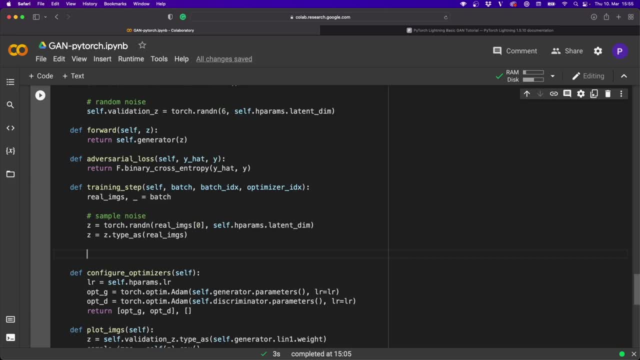 we can have this as the differentvia, in this case with dot h, but to put this back and on. So f of the global terms, you can save it x. All right, so we've got our shell here and everything here was free. We're just gonna store in reruns 아�K and yes. 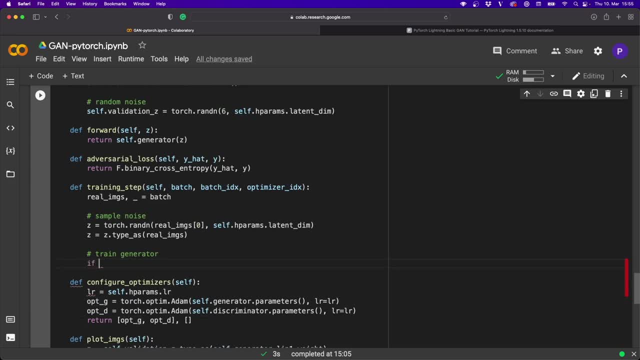 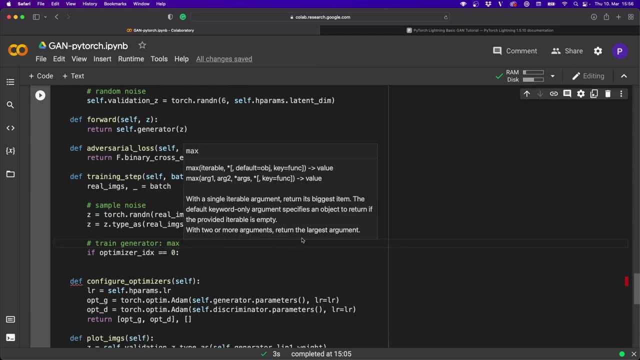 we want an out of the box component there, But what we're going to do is we just script deus, creative, high value terms in a dot st vault with the condition data work zero, unaenl, em discriminator, And here I will write the formula for you. So here we want to maximize the lock. 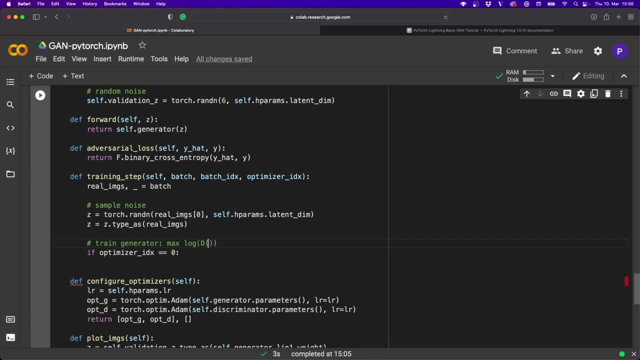 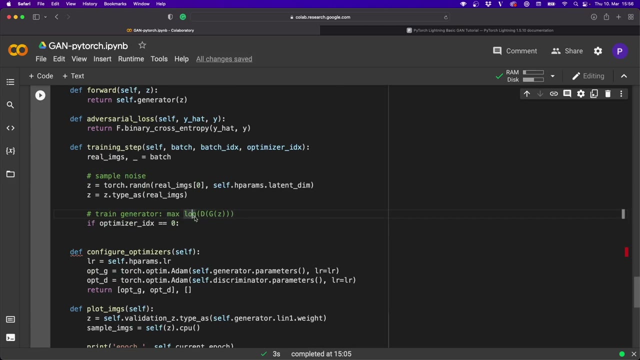 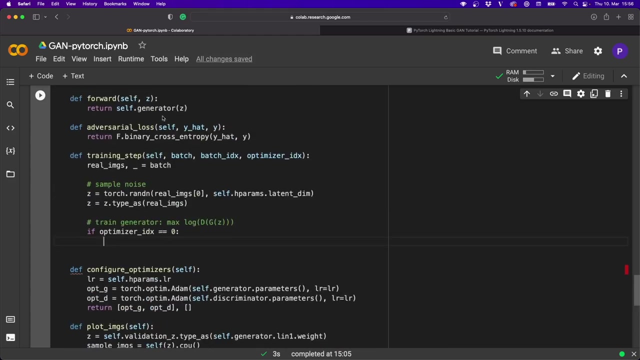 off, And here we use the discriminator, and then the generator of C and C will be fake images. So yeah, again, I will put a reference below the video where you can read more about the loss function. But yeah, this is basically the formula, together with this binary cross. 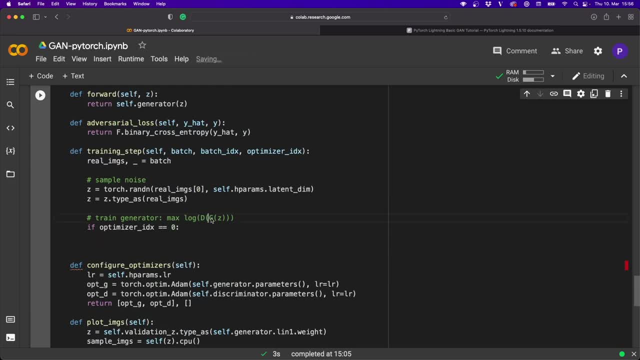 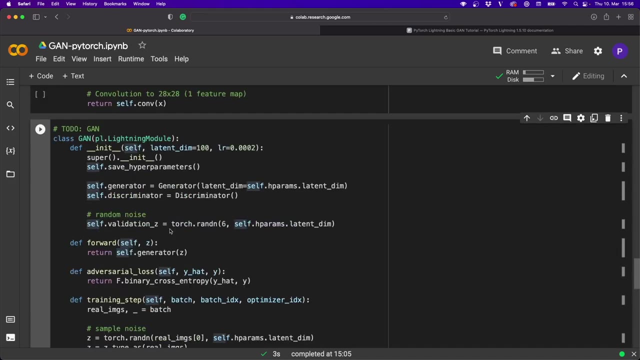 entropy loss. So let's do this. So first we want to call the generator with C, So we and this will be the fake images. So here we can call self dot C, So again, self dot C will execute the forward pass, which will execute the generator. 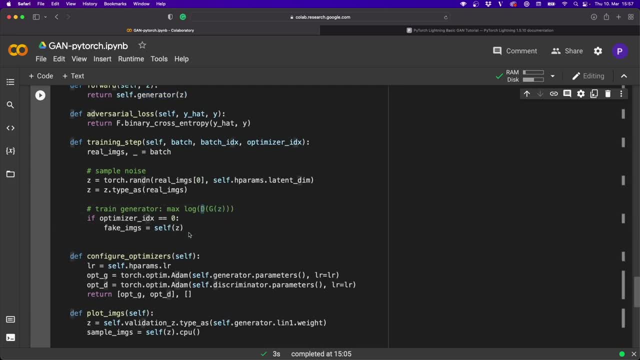 So this is this part. then we need the discriminator, And this will be the y hat, So the predicted labels. So here we call self dot this criminator, and we put in the fake images. And now, as real wise, so as real labels, we say y equals, and this will be a tensor of simply y equals. 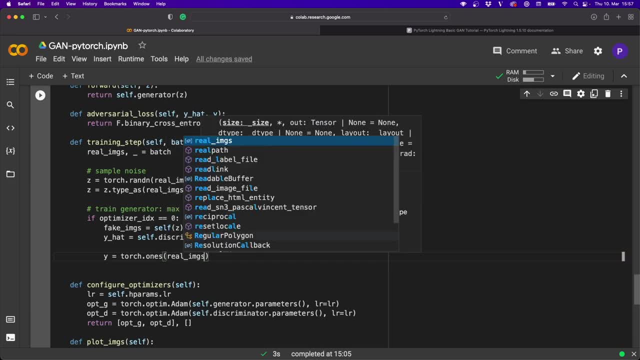 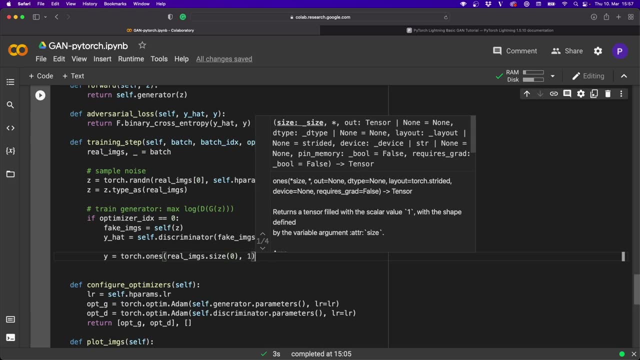 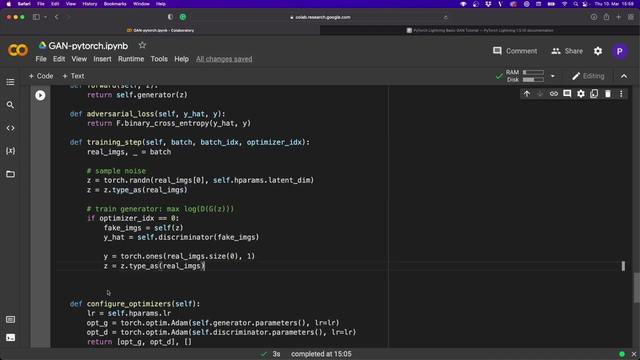 So we can say real images, dot size zero. and a second thing: we just say one, And then again we have to move it to the GPU. So again we can use type s. So here we say y equals y type as the real images, And then we create the or calculate the loss. So we create the. 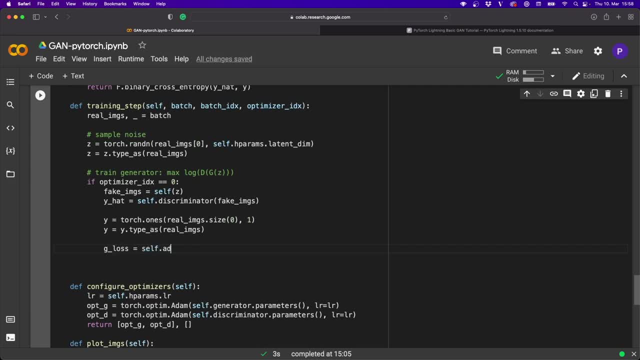 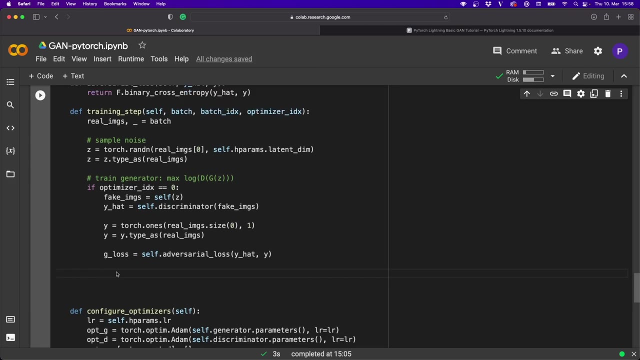 loss. we call this G loss equals self dot, adverse serial loss. so the function and this gets y, hats and y, And then we return this. So pytorch lightning knows what to do with this loss. So we create a lock dictionary And this is a dictionary with the value, with 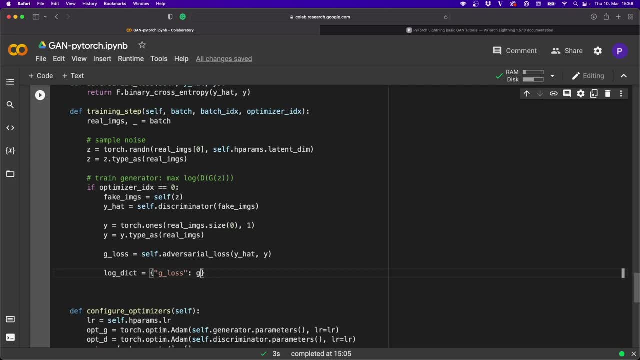 the key g loss and we put in the G loss in here And then we return a another full dictionary that this, that has this included. So first of all we need to have the key loss in here And the loss will be the G loss. then we can also say the progress underscore bar gets also. 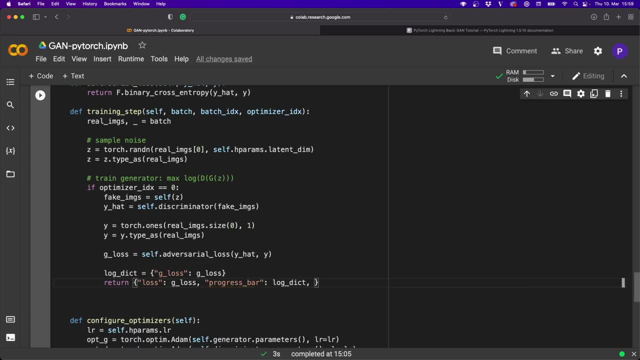 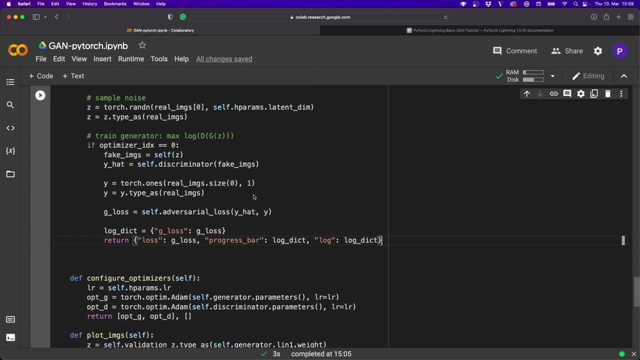 the lock dictionary And we for logging. if we want to use this later, for example in the tensor board, then we can also use this key And this also gets the lock dictionary. So yeah, this is what we have to do for the generator, And then we do a similar things. 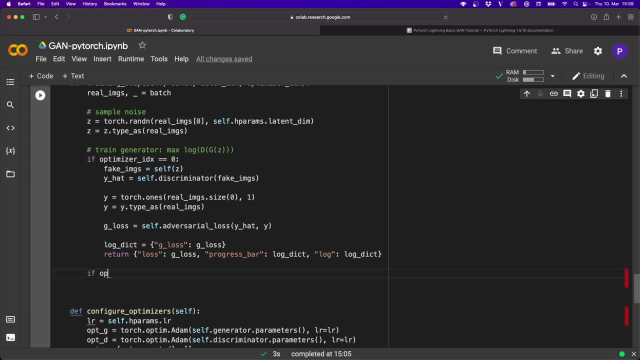 for the discriminator. So if optimizer in index equals equals one, And let's first write a comment here. So here we want to train the discriminator. And now again I will say what we have to maximize. So here we want to maximize the lock of D of x, and x will be the original images plus. and then here 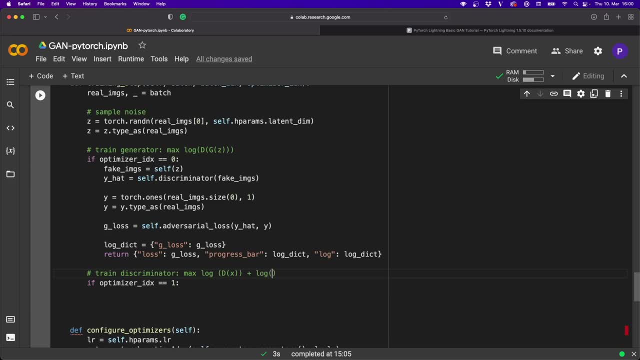 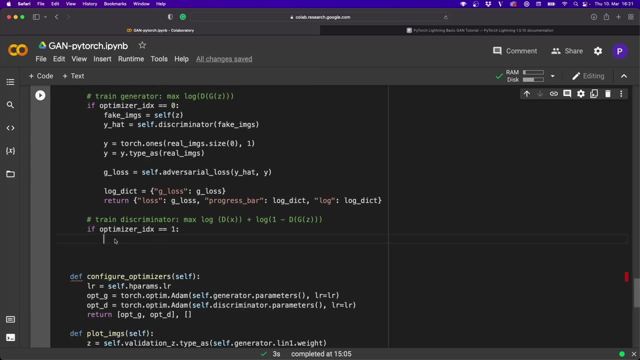 the lock of one minus D, of g, of C. So let's go over this and then it might become clearer what this means. So here we want to measure the discriminators ability to classify a real from generated images. So we want to check how well can it label as real? So how well? 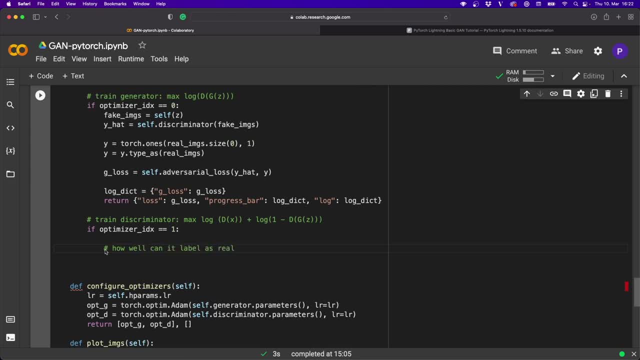 can it label as real? And then also, how well can it label the generated images as fake? And these are essentially those two parts. So for the first one the code is very similar to this one. So we create y hat real equals, and then we again self dot this criminator. 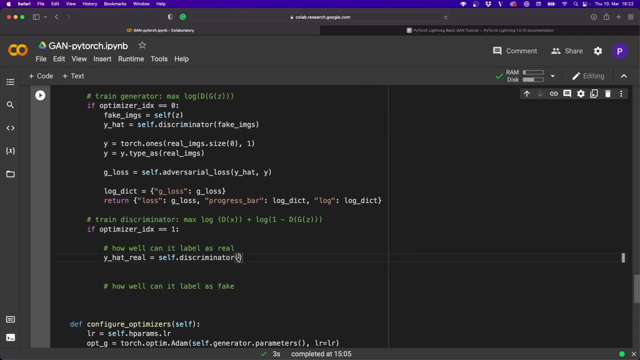 And now we don't put in fake images, But here we put in real, the real images, And this is the y hat real and the normal y real, So the actual labels. In this case it's also just torch dot ones like we use here, And then again we have to move it to the GPU if we 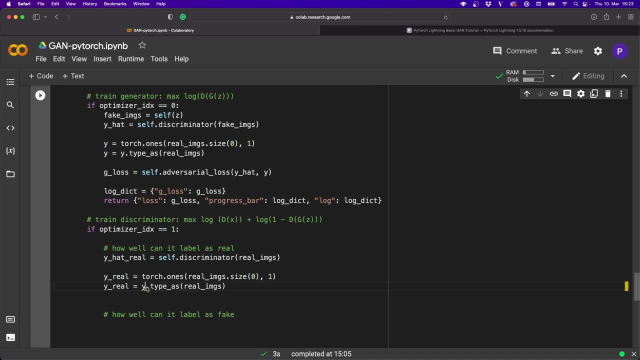 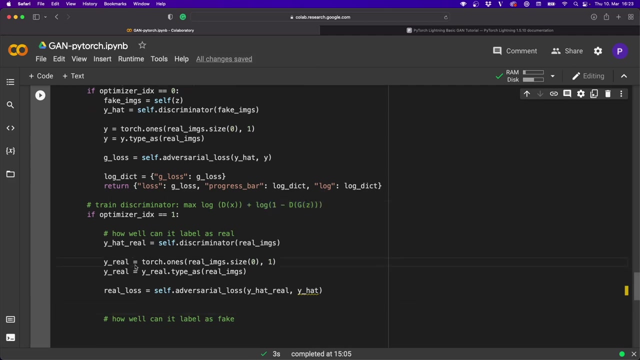 use one. So why Real equals y real type is real images And then we calculate the real loss: equals self dot adversarial loss of y hat real and y hat. So this is the first part. So this is very similar to here And now we need this part. 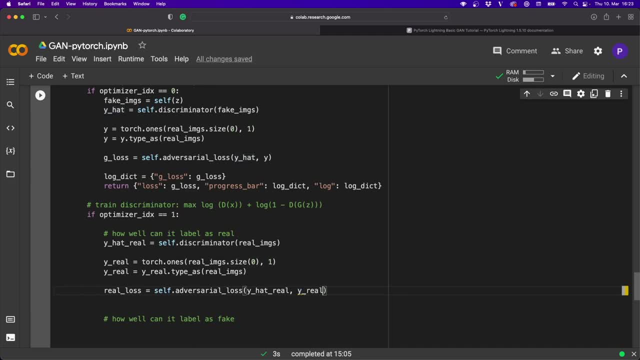 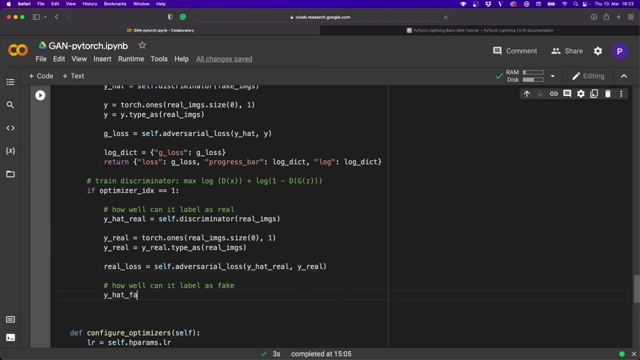 So here y real. And now how well can it label as fake? So here we call this: y hat fake. And then again self dot this criminator of self with C, And now we have to be careful. So self dot C will basically generate fake images. 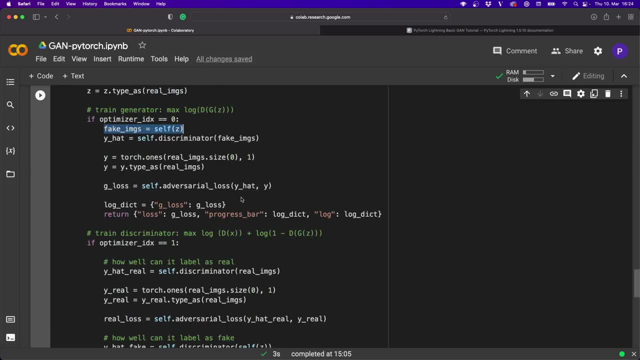 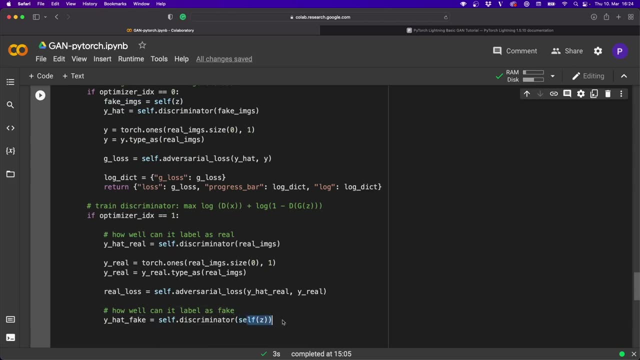 And we already did this here And we want to use the same ones here. But when we execute this, then this will do calculations on the graph And we don't want to do this twice. So that's why here we call C self, C dot, D touch, So this will create a new tensor that 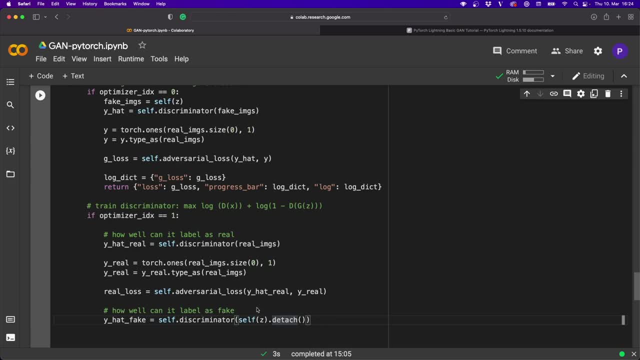 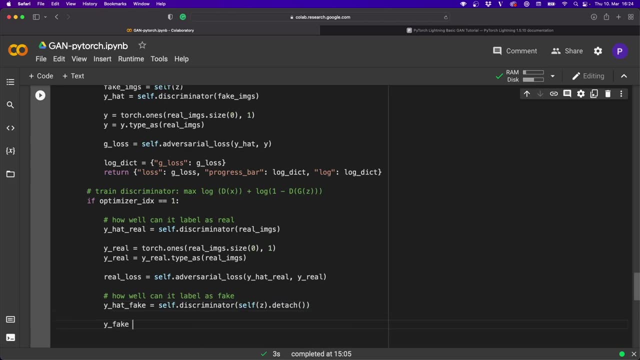 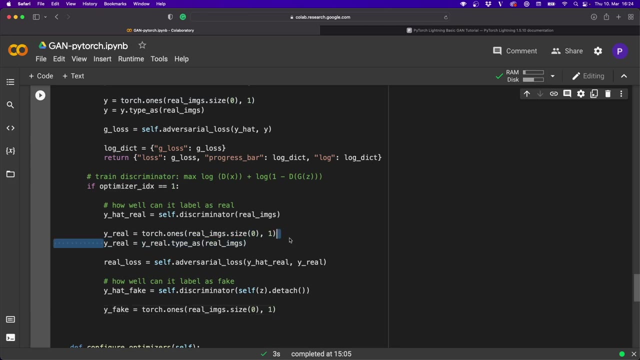 is detached from the computational graph. So be careful here. And yeah, this is our y hat fake, And then the y fake equals And this is very similar to here. So then again, we want to move this to the GPU. So why fake equals? why Fake? 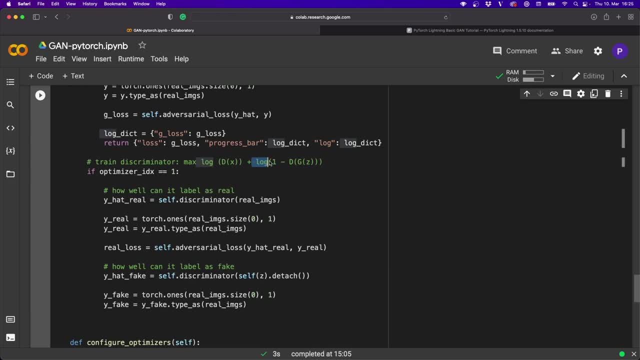 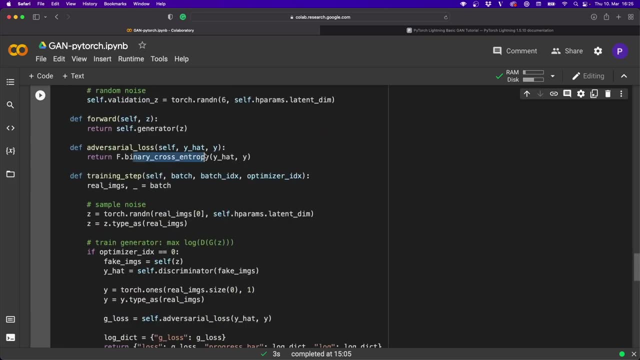 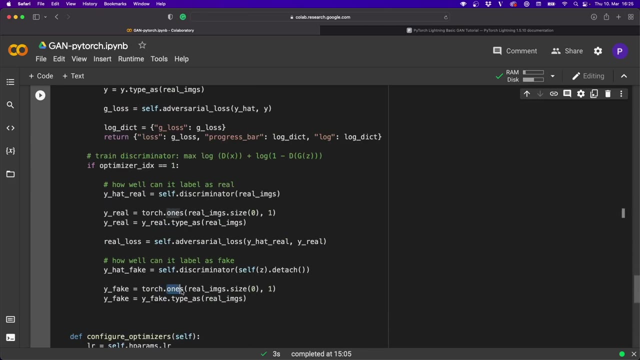 And now we have to be careful. So now this part says one mic. That's not a good sign. minus this. So actually, if we have a look at the binary cross entropy formula, then we find out that if we put in zeros here, then we actually end up with this formula. 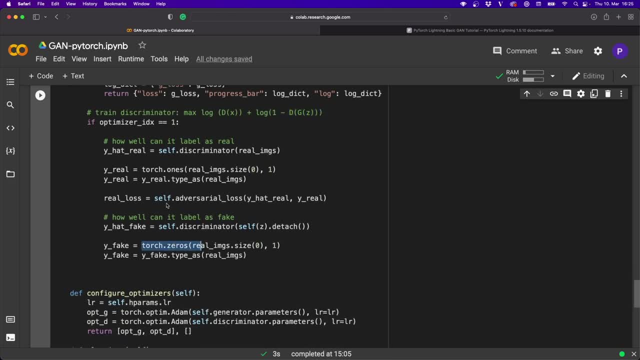 So here we put in torch dot zeros. So yeah again, I recommend that you just double check this for yourself. And then we also calculate the fake loss again with self dot for Sariel loss, And here we put in y hat fake and y fake, And then the total loss is the average. 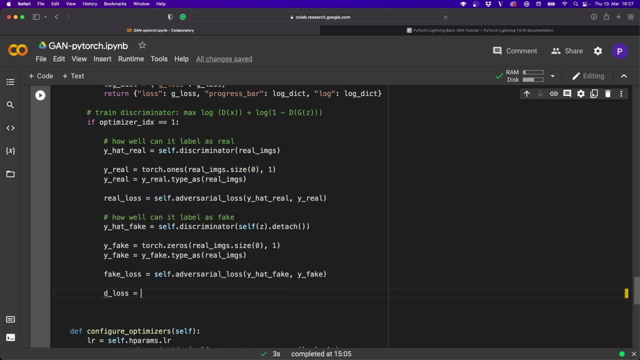 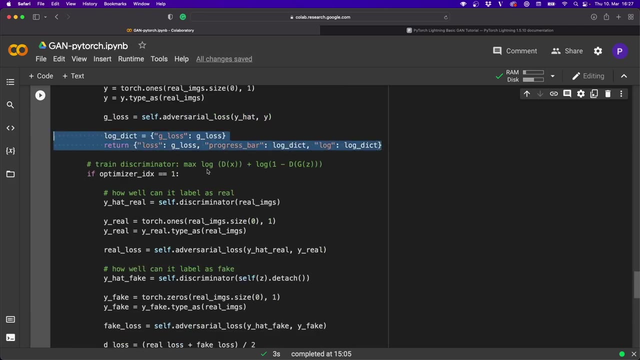 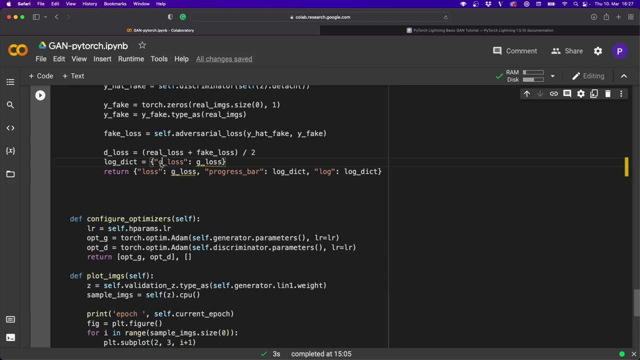 So we call this the D loss, So the discriminator loss equals, And here we say real loss plus the fake loss divided by two, and then the same as we do. here we create a lock dictionary and return this, and in this case we call this D loss and use D loss here and also here. 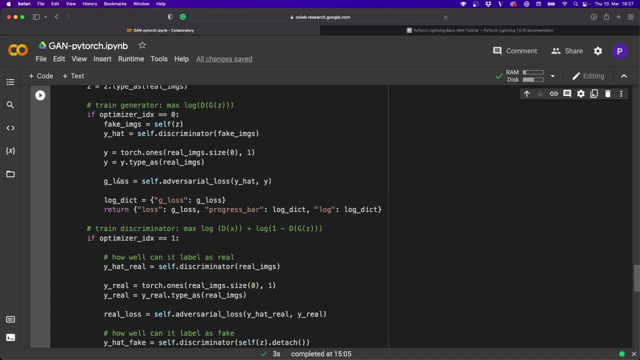 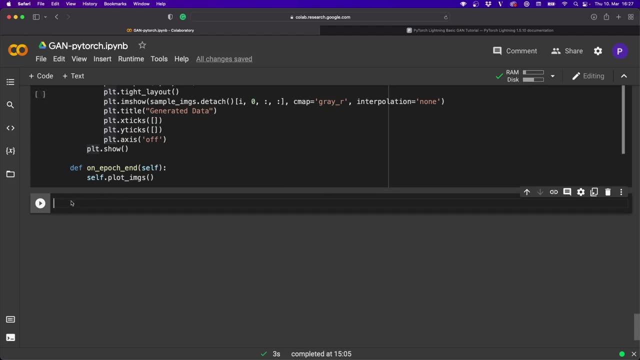 And now this is everything that we need for the training step. So let's create a new code, set cell. And now we want to set everything up. So we create a data module by saying: this is the MNIST data module that we created. then we create a model. So this is our GAN. 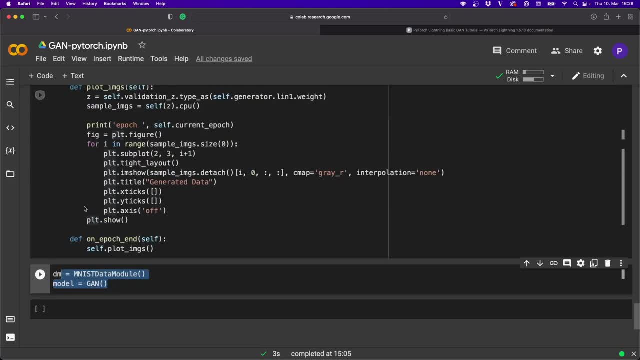 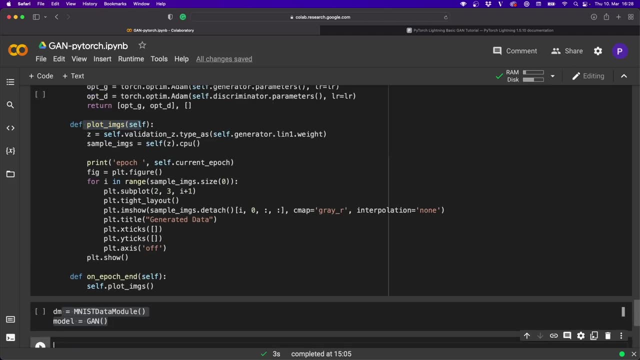 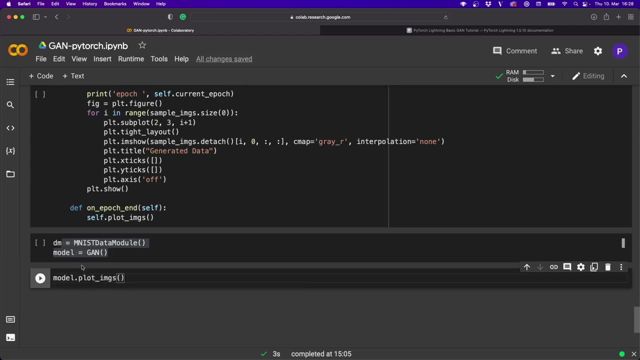 then again, and now, before I want to train this, I actually want to call this plot images one, so that we see that in the beginning we simply plot noise. So let's say model, dot, plot images, and then let's run everything and see if it works. until here, And yes, so. 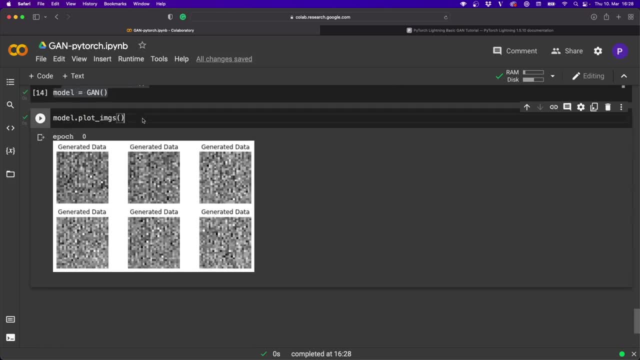 here we have the first generated images And, as we can see, this is just noise. And now we want to train our GAN, So we call a, we create a Python lightning dot trainer, And here we can specify the maximum number of epochs equals: let's. 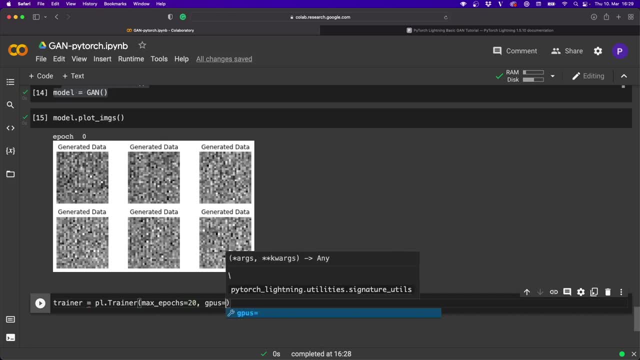 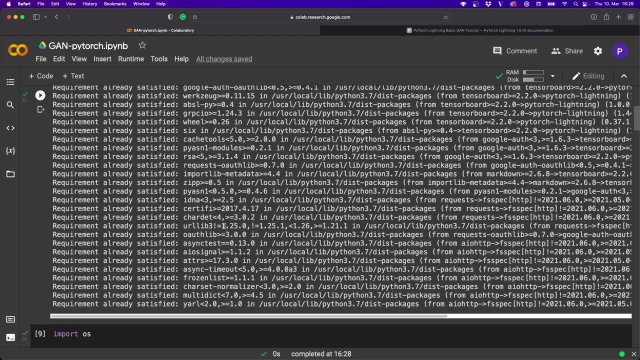 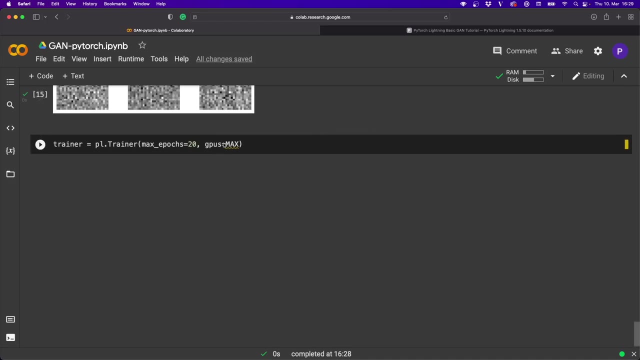 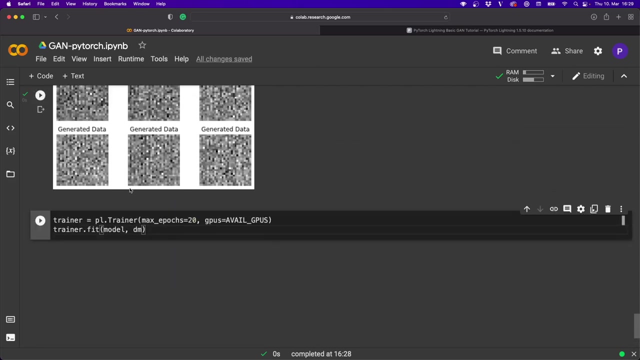 use 20.. And then we can also use the GPUs. equals the max. What would we call it in the beginning: max, no available GPUs. So let's put this also into our trainer. And then we simply say: trainer dot fit the model, And we also put in the data module, And then we 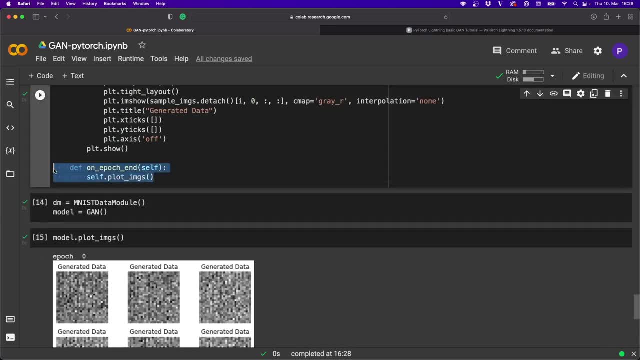 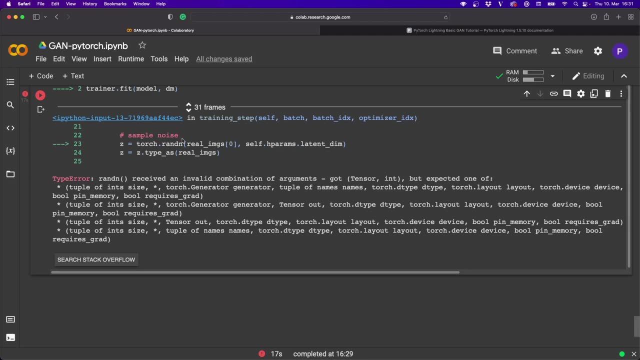 run this And when we execute this you might see that after each epoch we should print the images. So let's do this And we get a type error. So in this part I forgot to call shape. So here in the training. 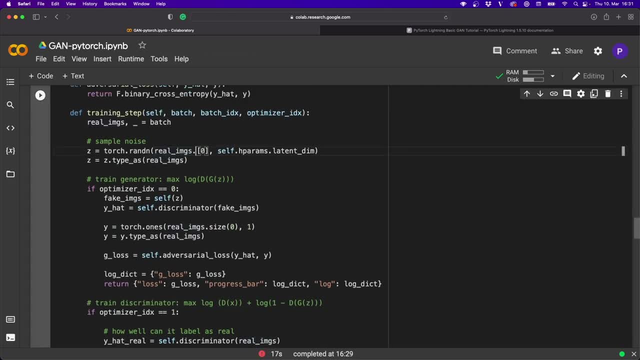 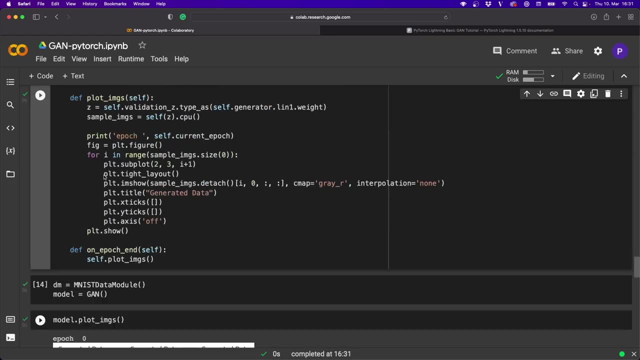 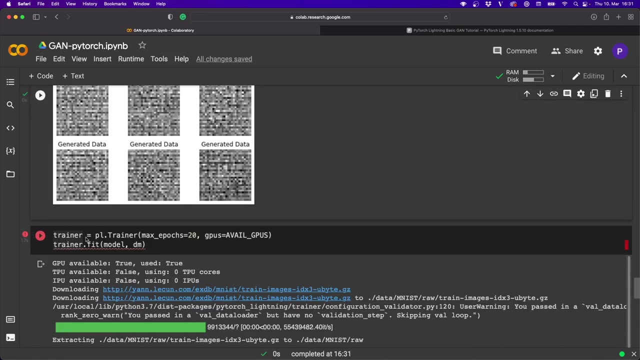 step we must say real images, dot, shape and then zero. So now again we have to run this cell. Then down here we again run this cell. let's again plot this. this should be the same random noise. And now let's run the trainer again, And training is done. 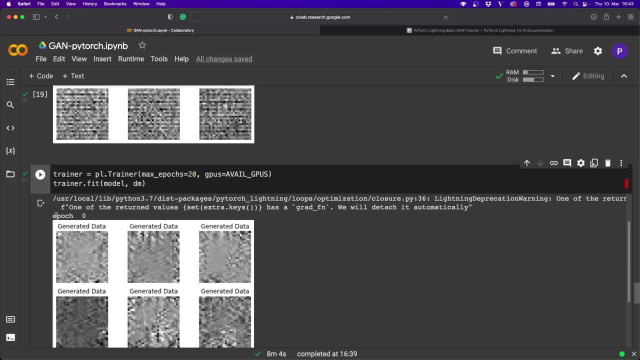 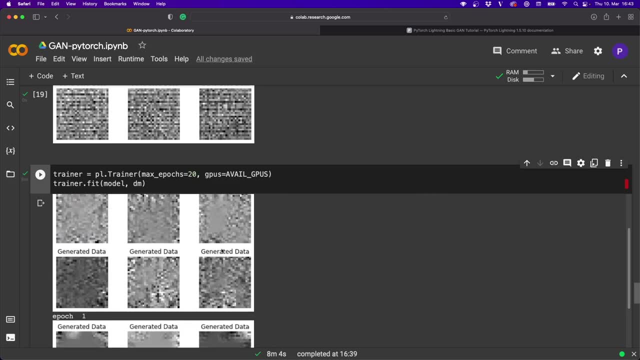 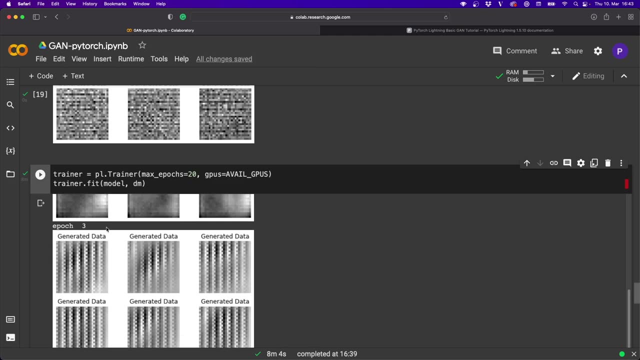 So now we can scroll down and see after the first epoch, So this is actually. Yeah. after epoch zero, we get this images, So it still looks like random noise. epoch one: we have this images, then this: it still looks like noise. But then after epoch four, it starts. 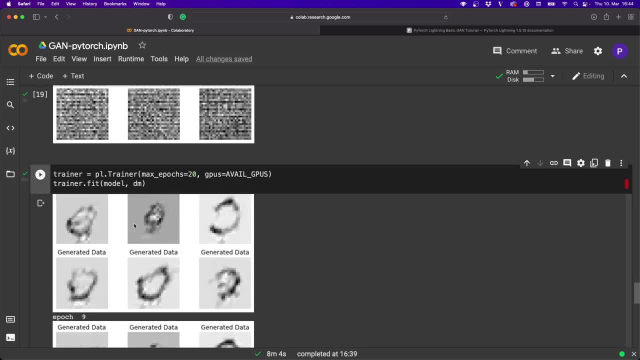 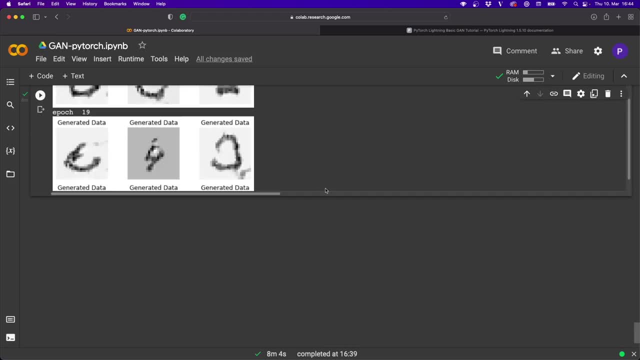 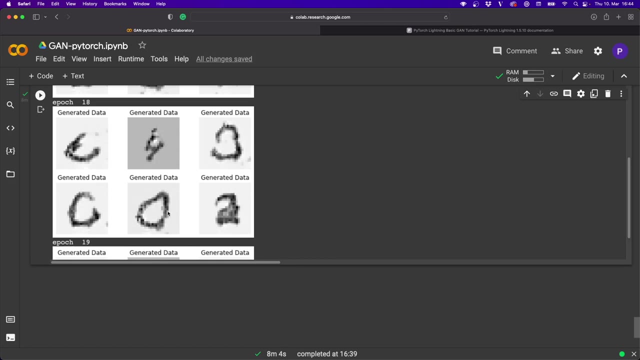 getting better And it's starting to look like images. So now let's scroll down a little bit, And yeah, so here it's still looks a bit noisy, But, for example, this might be a three, this might be a four, this might be a zero. So, yeah, it's starting to get into shape. 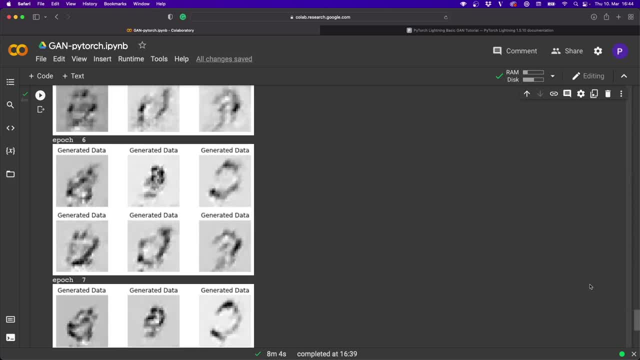 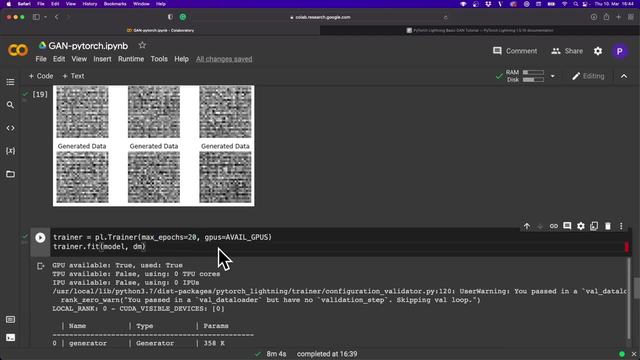 And, yeah, our code works And yeah, I actually recommend you that you play around with the hyper parameters a little bit and also maybe increase the maximum epochs And then test this for yourself Again. the call up will be the link to the. 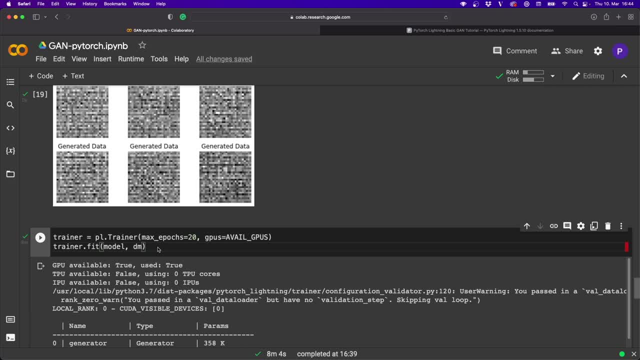 call up will be in the description below. And yeah, I hope you enjoyed this video. If you did so, then please hit the like button and consider subscribing to the channel, And then I hope to see you next time. Bye.